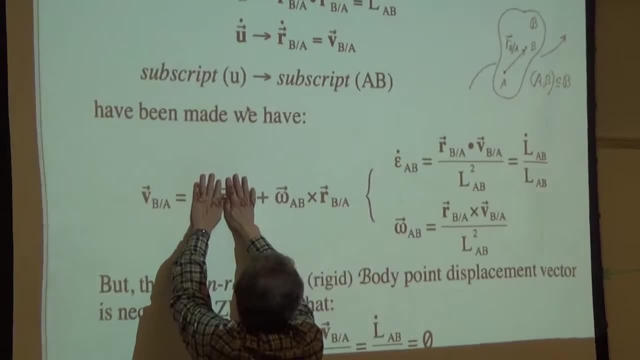 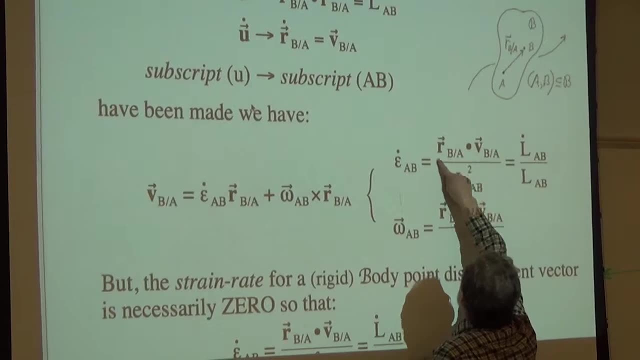 would have to be zero, which tells us that this term can't be there in this application. Well, since that is zero, this is zero, making this zero, and that gave us our final result, Our first extra bit of information. So we learned right away that, for any two points, 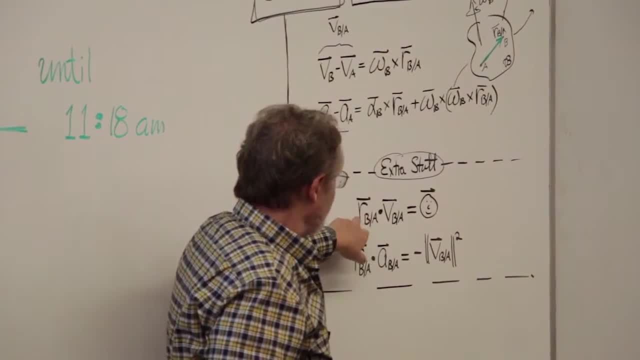 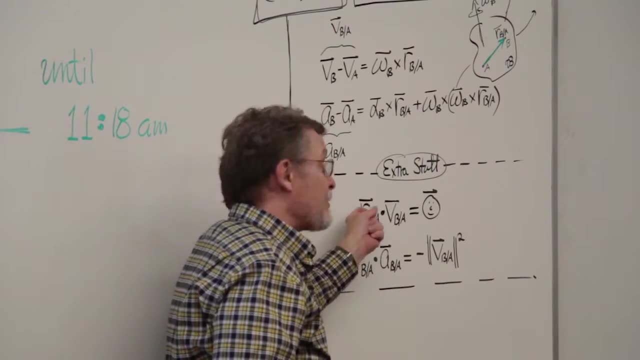 any two points, any pair of body points, the relative position vector between those two points, dotted with the relative velocity between those two points, has to be equal to zero. It's just an affirmation of the fact that that length of that body line segment must. 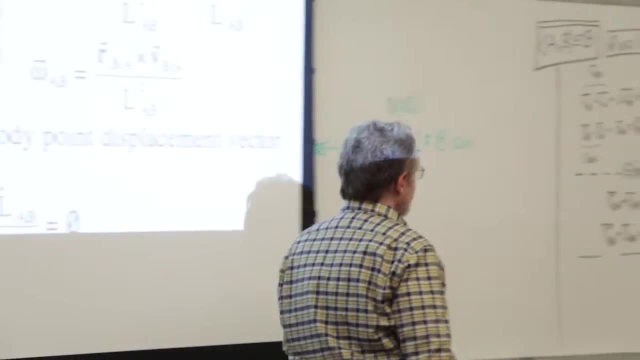 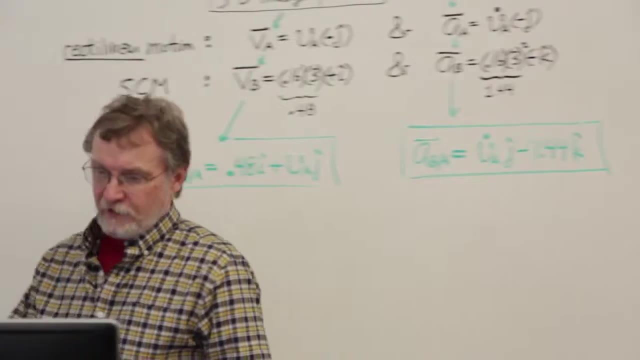 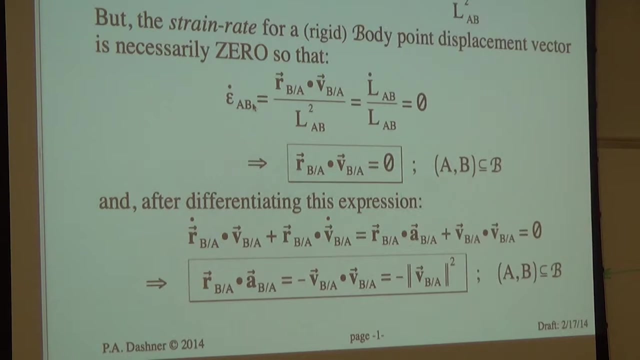 remain constant. And then, of course, if you took a time rate of change of this, make a time rate of change of that expression which we did below, you come up with that second little extra bit, And that's just a straight derivative of the line above. Now, that's great, So we've got. 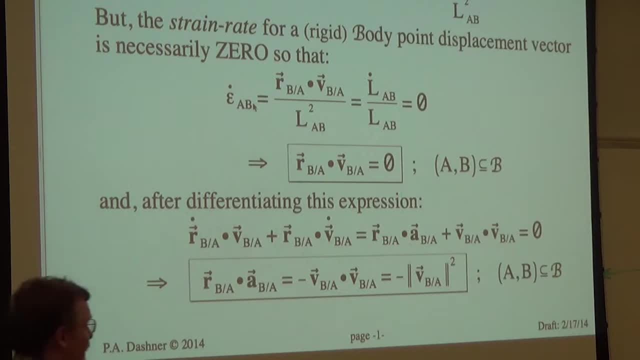 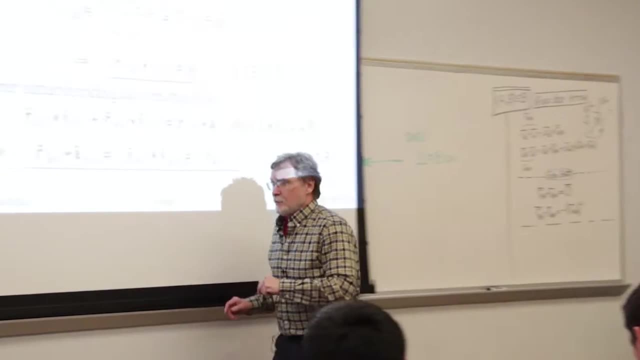 a couple extra little things. We've got these two little scalar dot product equations which are supplemental to what we knew before, And our first application of this was to that three-dimensional linkage. It's a nice little application As a matter of fact, those equations. 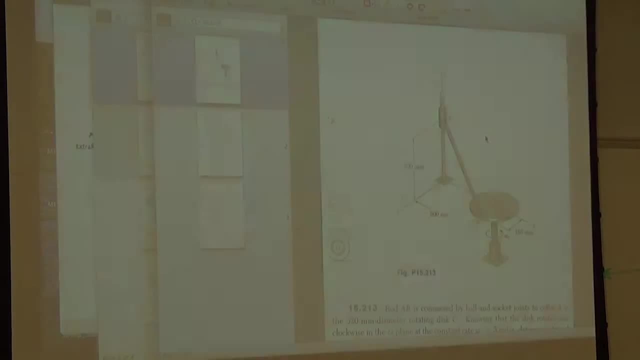 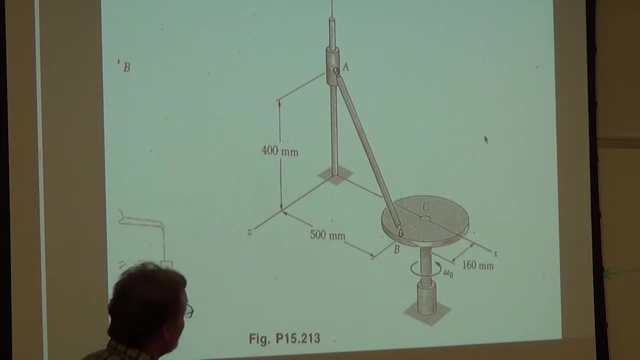 really come in handy whenever you deal with three-dimensional linkages. So this was the problem we looked at. We were given that this link AB was ball and socket connected to a disk and to a collar which could ride on the vertical pole. We were told 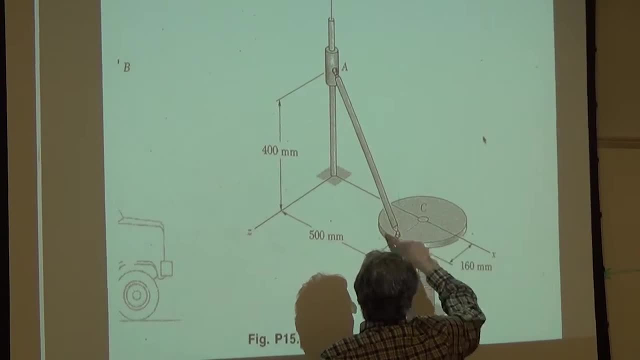 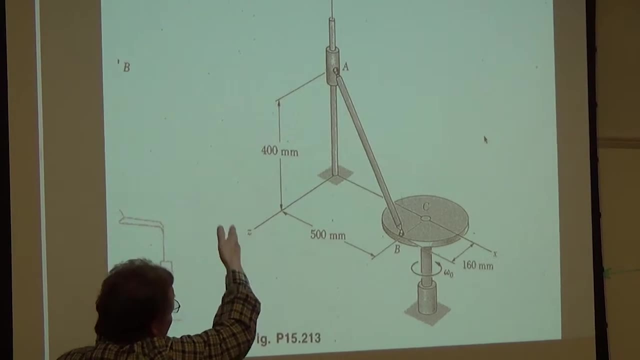 that this disk of radius 0.16 meters was rotating at a constant speed of three radians per second, And we said, okay, what do they want here? First of all, it was clear to everyone that point A is moving with rectilinear motion in the vertical direction. And then at this: 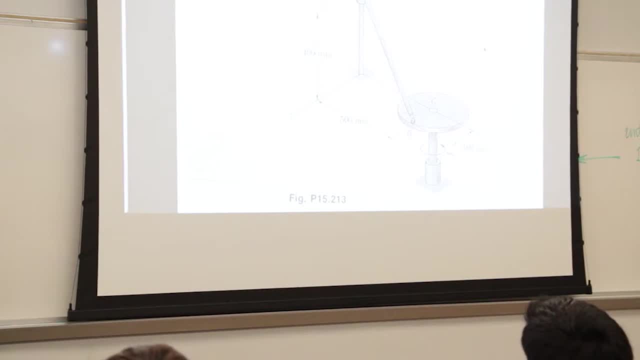 moment it was moving in the vertical direction, And then at this moment it was moving in the vertical direction And then at this moment it was moving downward. So I think you could all say, just by inspection, that since A has rectilinear motion, its velocity vector would: 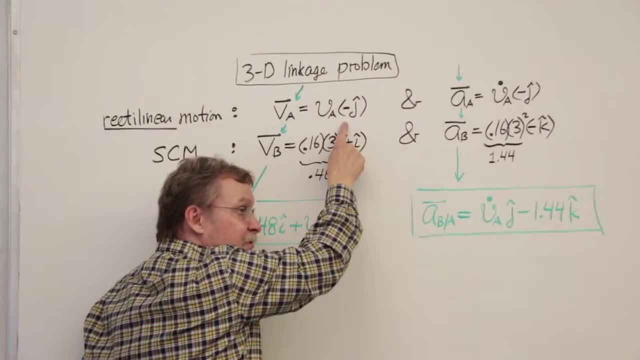 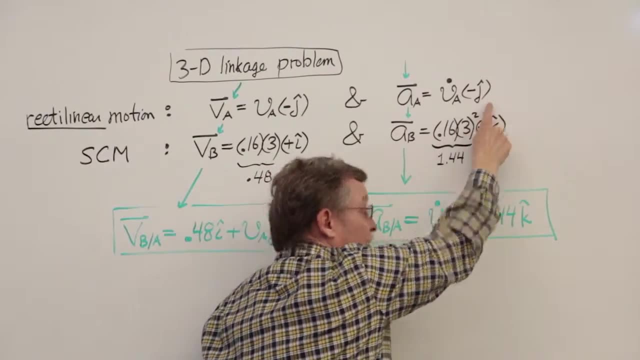 be its speed in its instantaneous direction of motion, tangent direction to its path. And because it's rectilinear motion, the acceleration would just be the rate of change of speed in the tangent direction. There would be no V squared over rho in the inward pointing normal. 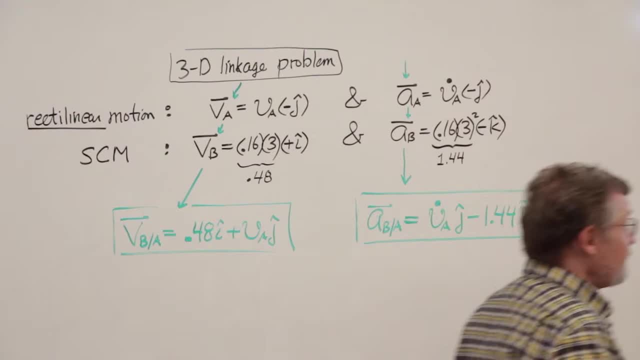 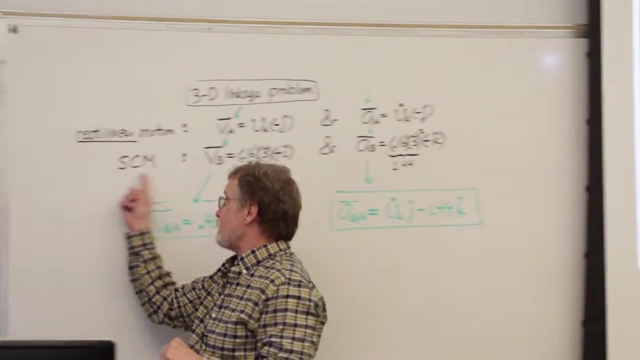 direction. You don't have that for rectilinear motion. On the other hand, if you look at the point B, point B has a constant speed of three radians per second And then at this point point B has another special kind of motion that I refer to as what SCM stands. 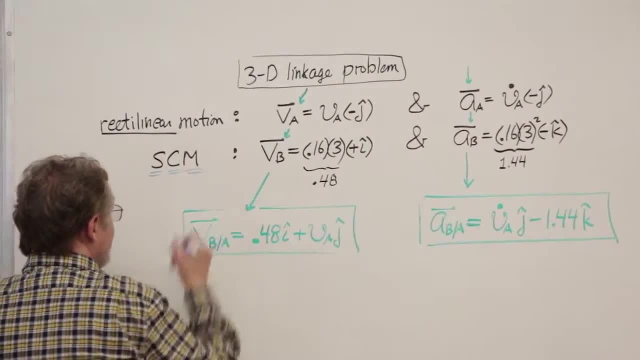 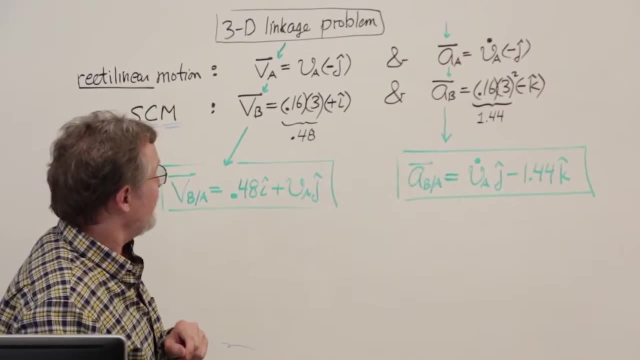 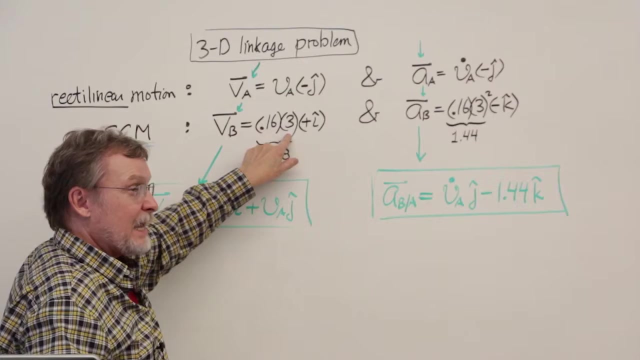 for simple circular motion, something that I hope you used in the quiz problem that you just completed, Because point B obviously has simple circular motion- pretty much by inspection. you can write its velocity vector: Radius of the path, angular speed around that path in the direction tangent to the path, And similarly the acceleration would be r. 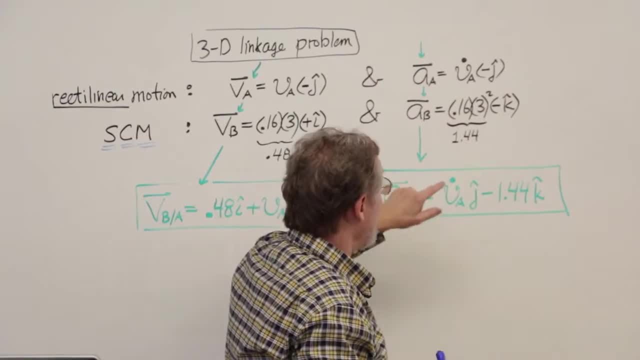 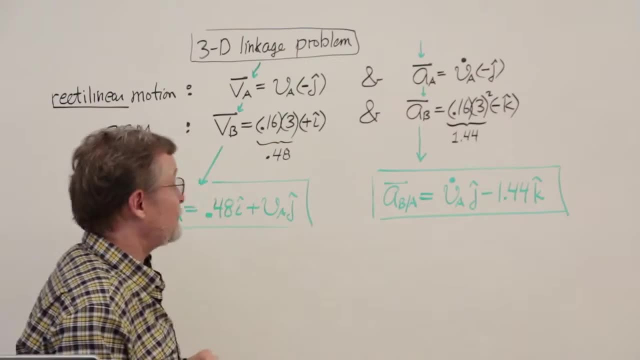 alpha around. well, it's constant omega. so there wouldn't be any of that. You just have the r omega squared pointing in towards the center of the path. So by inspection you can figure those two things out, And then, of course, remember what is the relative velocity between. 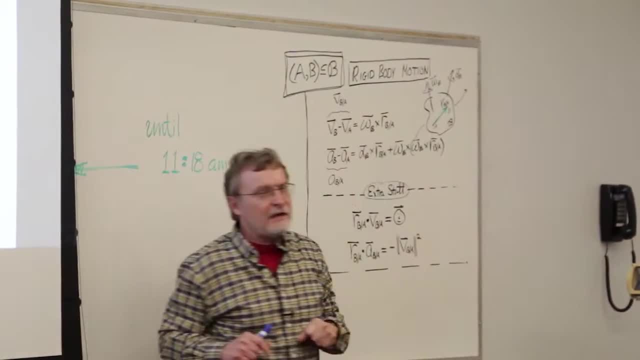 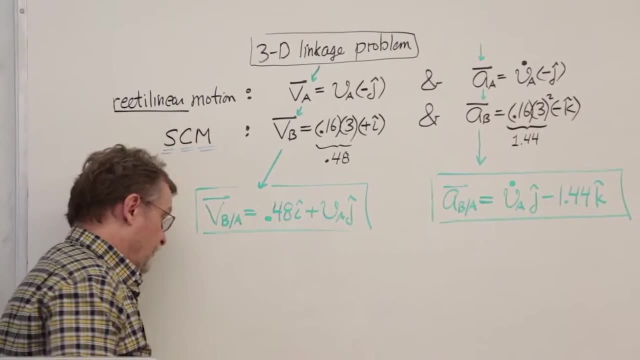 those two points. Well, it's the difference of velocity, It's relative acceleration, it's the difference of the acceleration. So from those observations you can quickly write down this expression for the relative velocity of those two points. The only thing we don't: 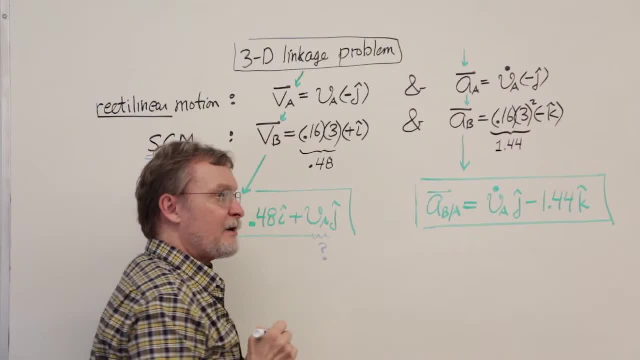 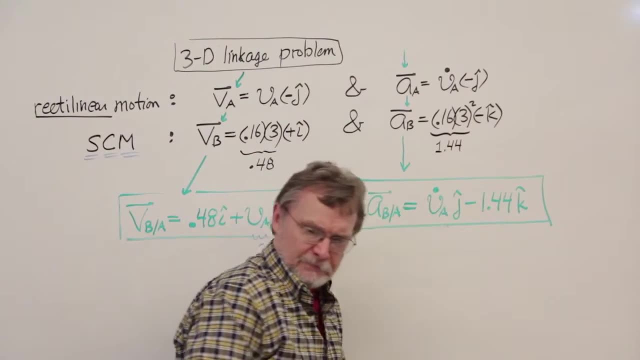 know there? we don't know the speed of A. In fact, that's what they wanted us to do in part A. They wanted us to figure out: how fast is the collar moving. So that's your first unknown. And the second part of the problem they wanted to know is that collar 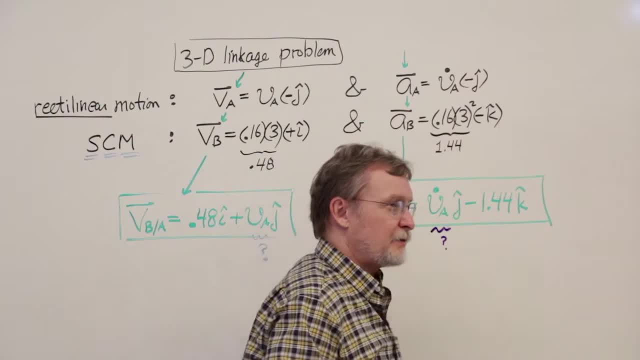 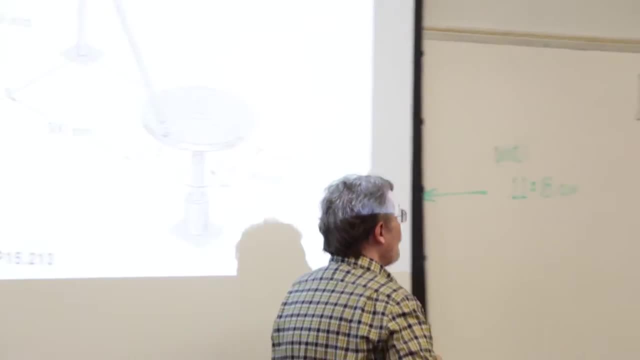 speeding up or slowing down, and at what rate. So those were your two unknowns: The unknown in part A, the unknown in part B. Two unknowns, one, two equations. So all you have to do to make things go from there is write down an expression for the relative velocity of 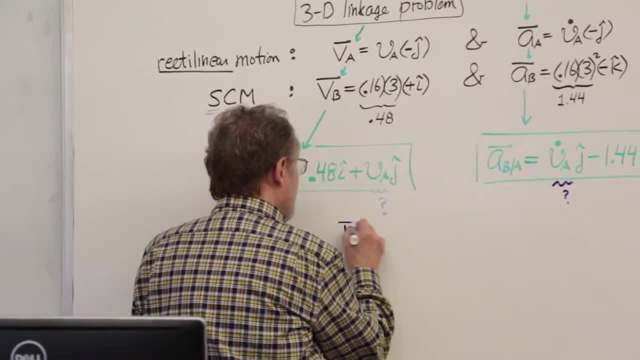 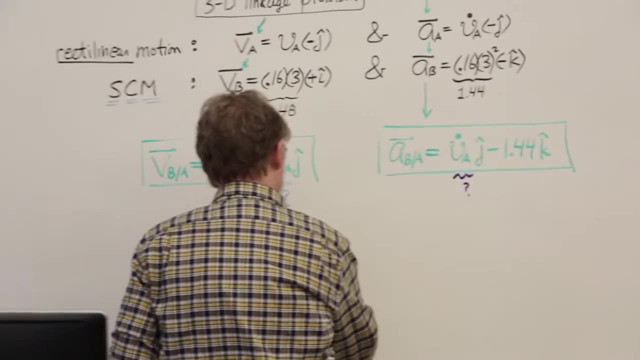 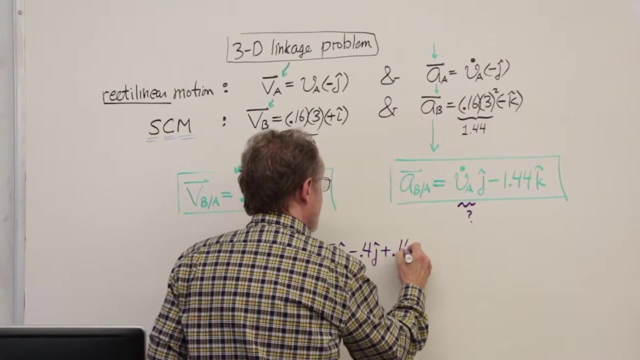 those two points. Here's an expression for the relative position vector, which we did. It's pretty obvious that to go from A to B, you're going to have to go half a meter in the I direction. You're going to have to go negative 0.4 meters in the J direction and plus 0.16 meters in the 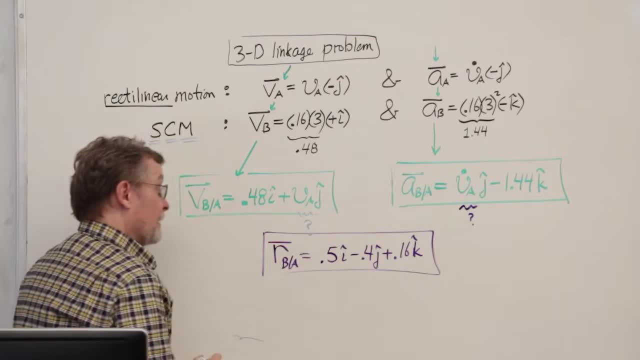 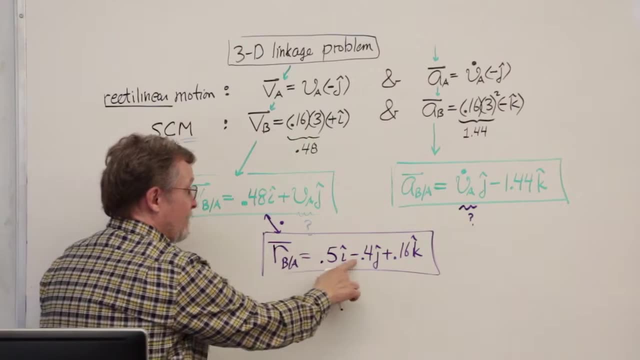 K direction. So all you got to do is set it up In A part. you want to dot these two vectors together- Trivial 0.5 times 0.48 minus 0.4 times VA- And then you're going to have to. 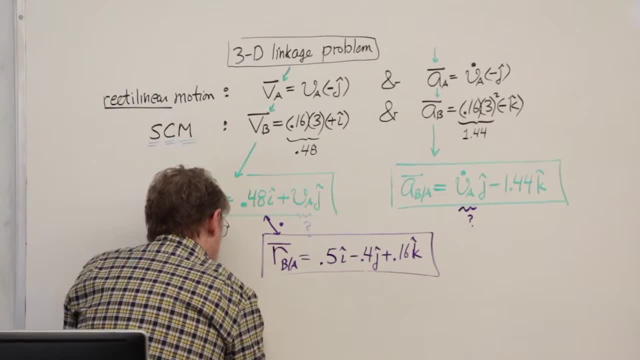 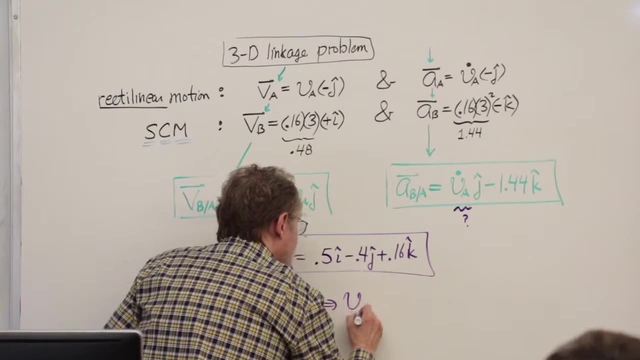 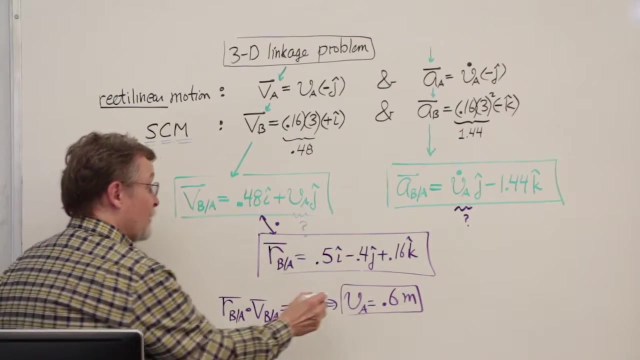 write down an expression for the relative speed of A equal to 0. And you can solve that: RB slash A dotted with VB slash A equals 0. Solve it and you get that the speed of A is 0.6 meters. By the way, once you've solved part A and once you know the speed, 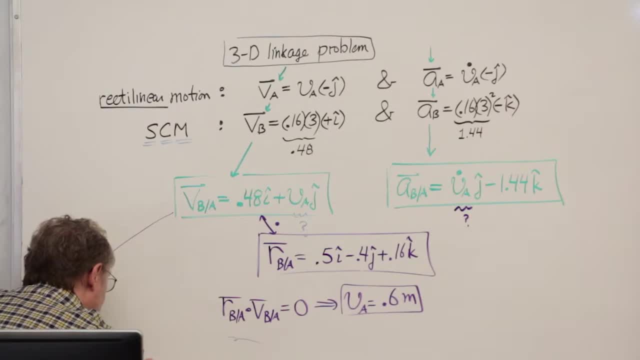 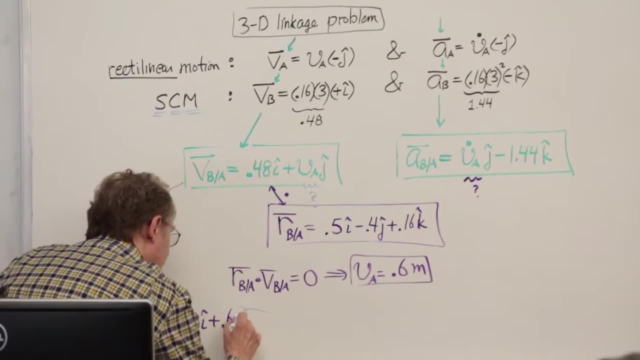 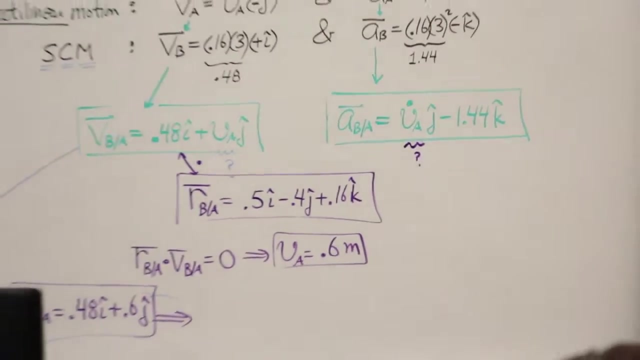 of A, then you would know that the relative velocity vector is in fact equal to 0.48i plus 0.6j. And why is it important that we know that? Because, to use this next equation, we need the square of its magnitude, because minus the square of its magnitude goes on the right. 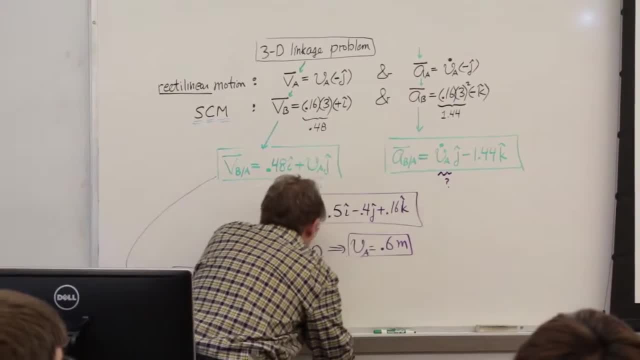 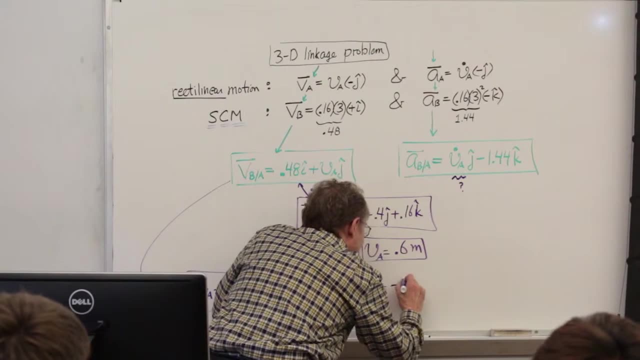 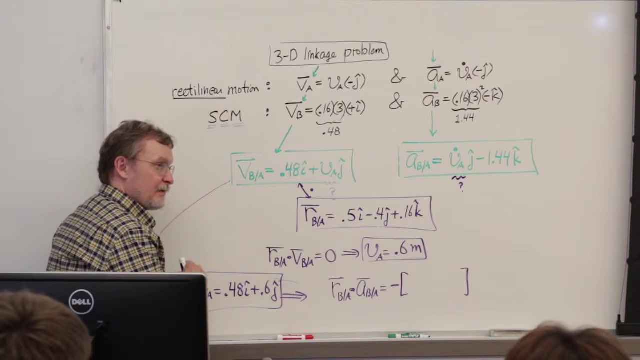 hand side of the equation. So when you set it up you're going to go like this: RB slash A dotted with the acceleration of B slash A equal to minus the square of the magnitude of this vector: 0.48 squared plus 0.6j. 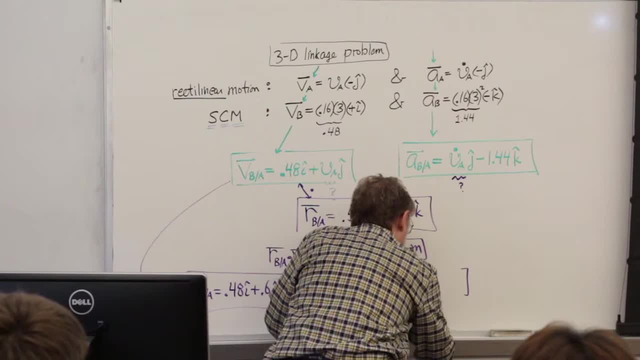 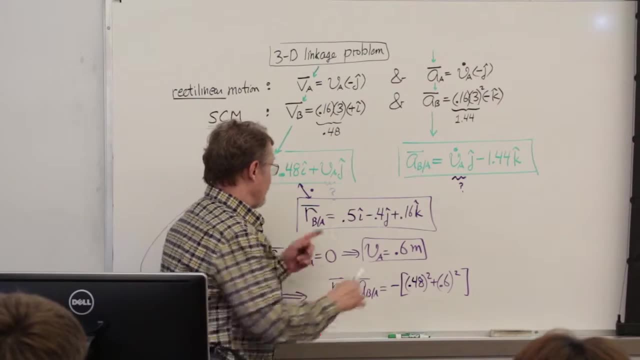 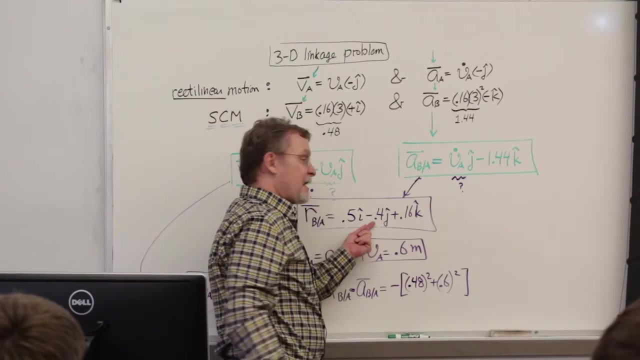 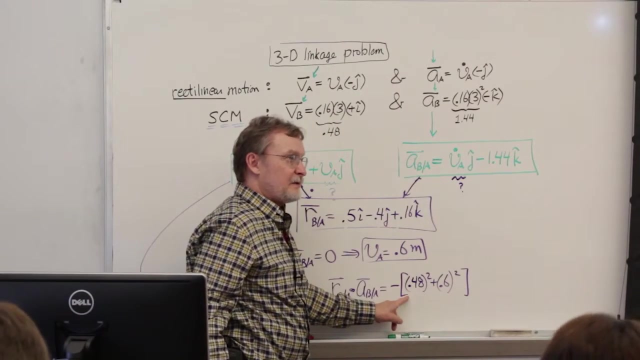 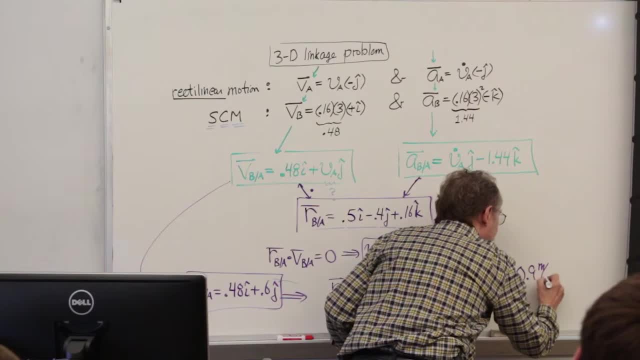 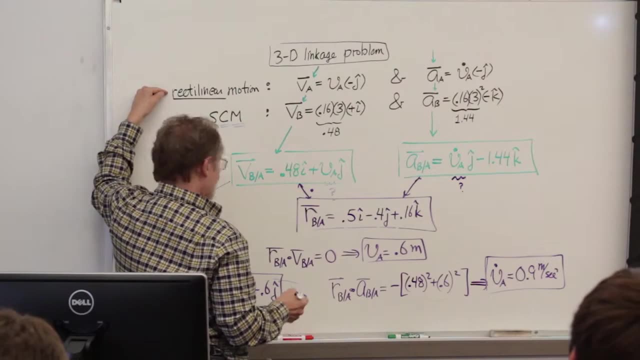 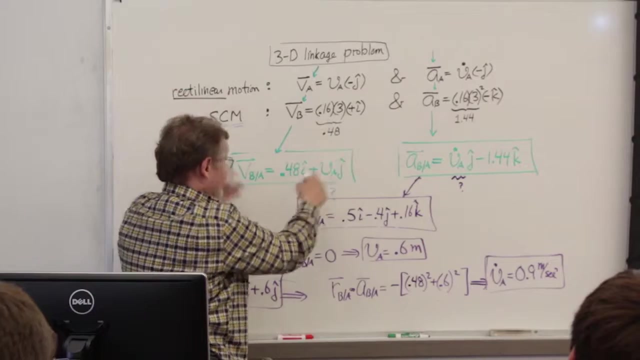 This comes out to be 0.9 meters per second squared. So we just make some simple observations related to simple kinds of motion. We understand rectilinear motion. We damn well had better understand simple circular motion and just make some observation. some simple observations. 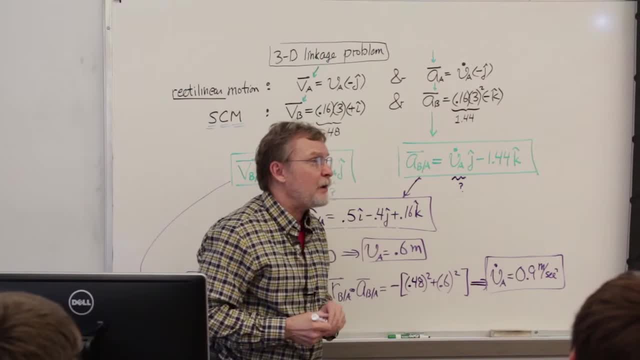 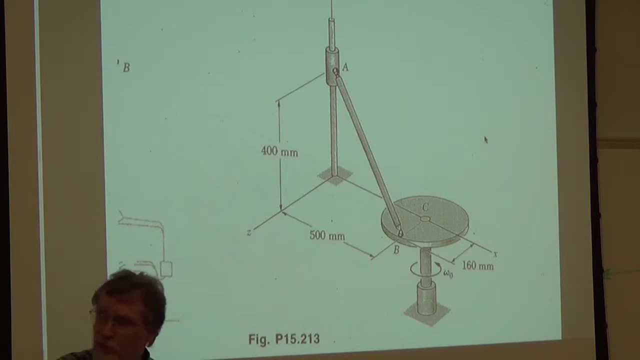 and plug into those two equations and we get what we wanted. Okay, And of course, the details are published. Now, if you look at the solution, you'll find that, looking at theğı, that this part of the solution only comes up on page two of the solution. 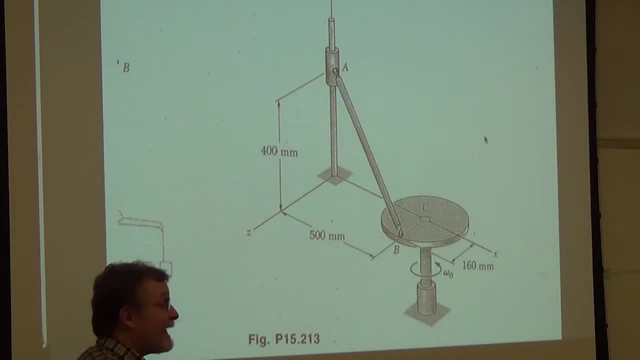 Because the first thing I set up was what Beer and Johnson actually had in their solution manual. I don't recommend that you do it the way he did it, but let me explain how he did the problem, Because some interesting things come out of this. 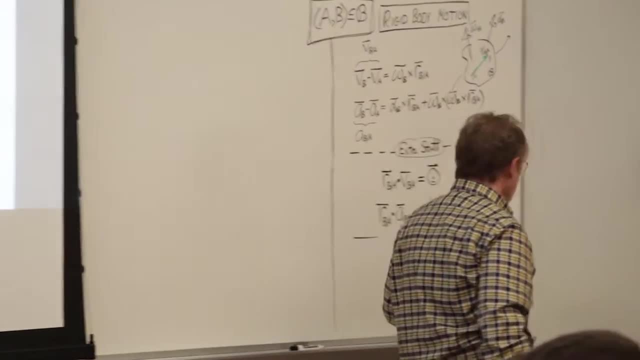 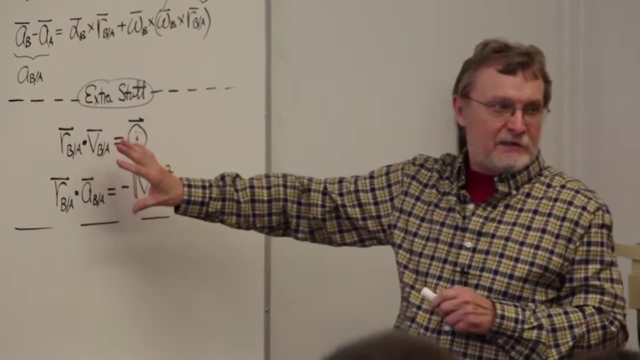 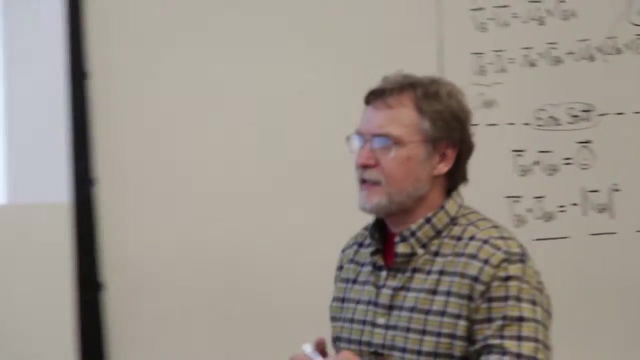 Apparently, at that point in his textbook, the authors Beer and Johnson had not exposed their students to these equations, So they didn't know about these equations. All they had was this: okay, Now I presume that when he set this thing up, 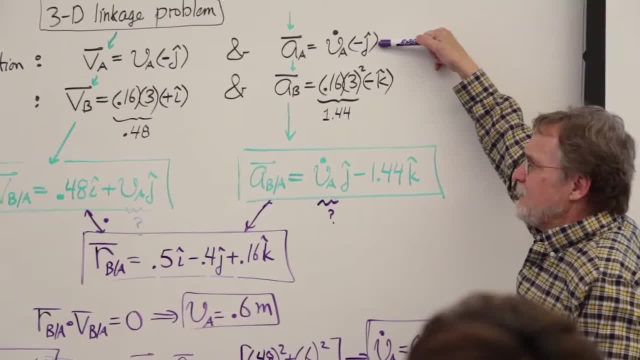 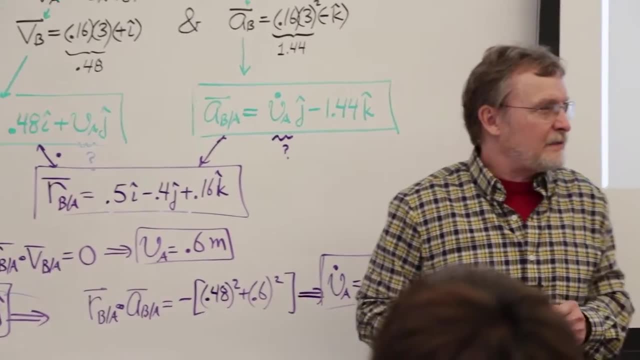 he did, his students did understand rectilinear motion and they did understand simple circular motion. so I think they'd already come to these conclusions by that time. But remember, he didn't have the dot product equations. He only had was the vector equations. 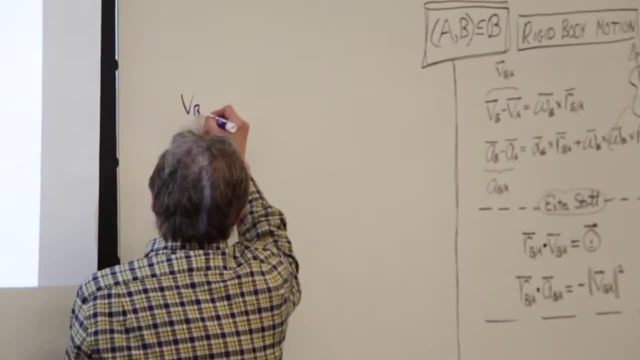 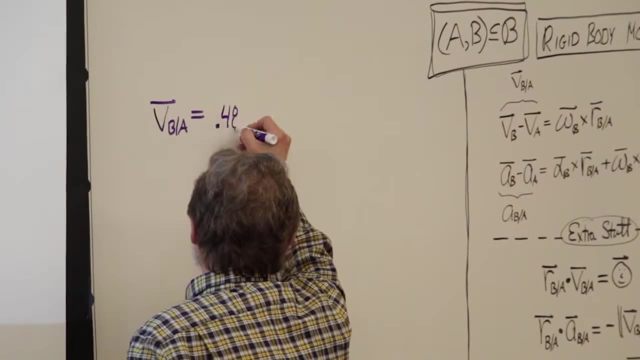 So what he just set up was this. He said okay. well, he said we, you know, if we start, if we look at this, if we look at the rectilinear and the circular motion, we can figure out that VB slash A is .48I. 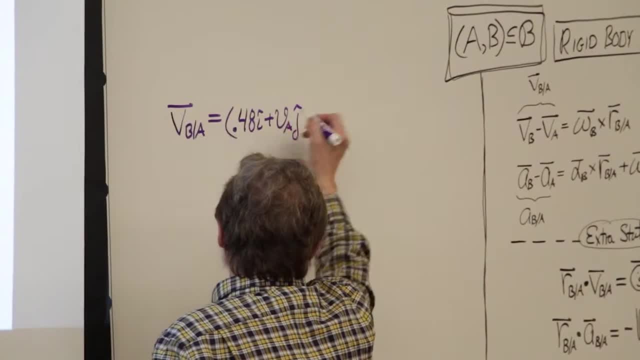 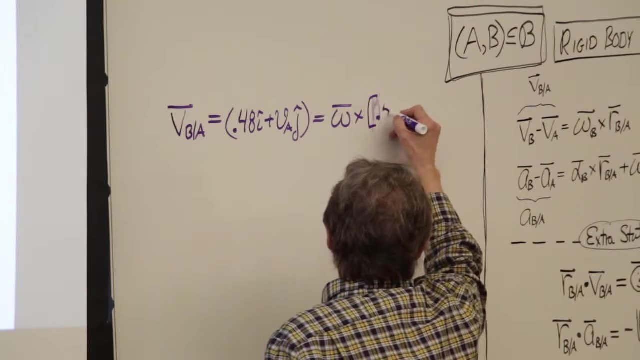 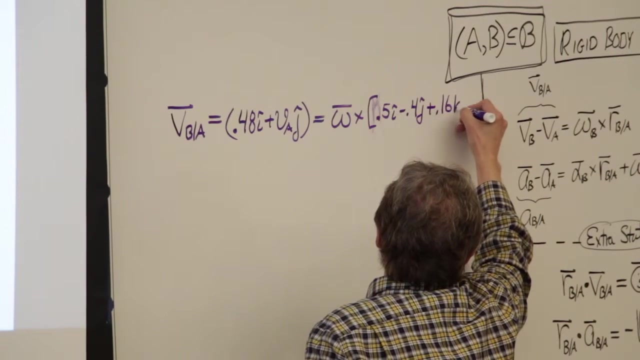 plus the thing VA, the thing we're looking for. There's our primary unknown right there And this is gonna equal omega crossed with RB slash A. And remember RB slash A, we figured that out: .5I minus .4J plus .16K. 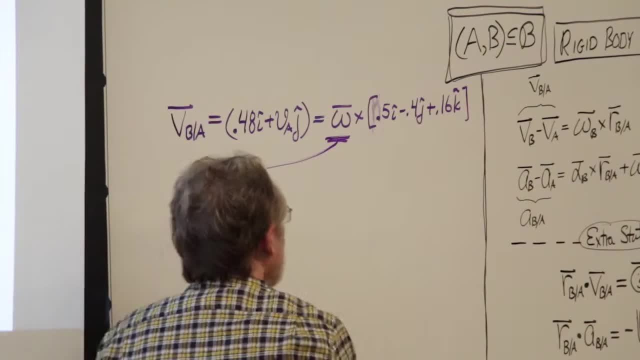 So he basically set up this equation. Now, in this equation, remember what omega would have to be: .5I minus .4J plus .16K. So he basically set up this equation. Now, in this equation, remember what omega would have to be. 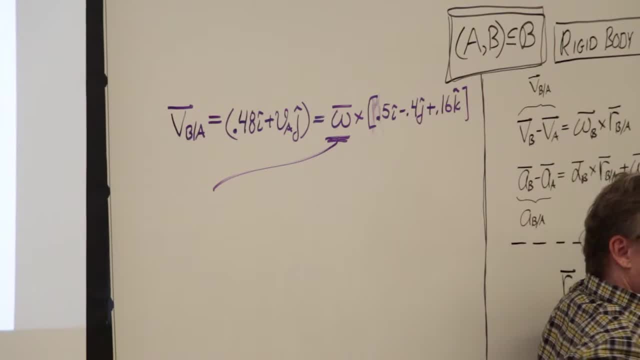 .5I minus .4J plus .16K. So he basically set up this equation. Now, in this equation, remember what omega would have to be. He's using this equation, so omega that he's talking about there would have to be the angular velocity of the link, right? 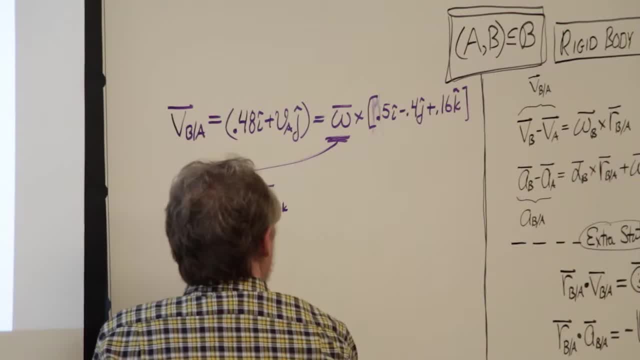 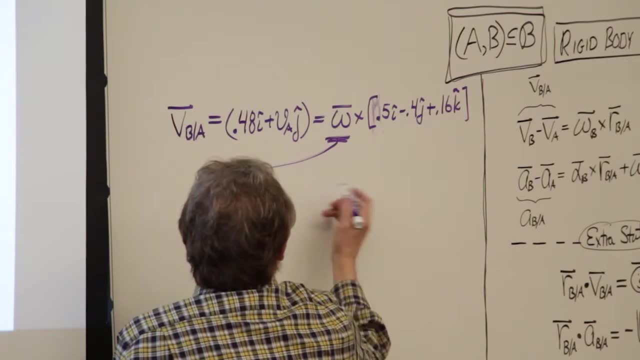 So you know, to give it a more precise name, I guess you could call it omega sub link, or you could call it omega sub AB, I guess. Well, let's just leave it at omega of the link. And, by the way, what would he know? 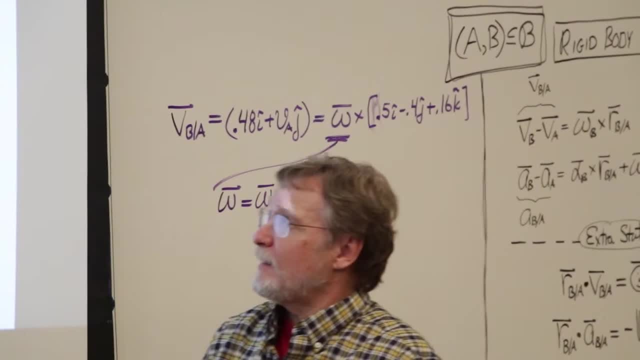 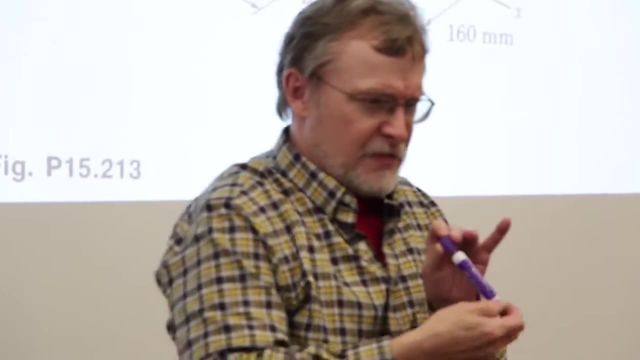 At this point, looking at the problem and reading the problem statement, would we know anything about the angular velocity of the link? The link, one end of it's moving vertically and the other end's moving in a circle. That's even. it's kind of hard to even, you know, imagine. 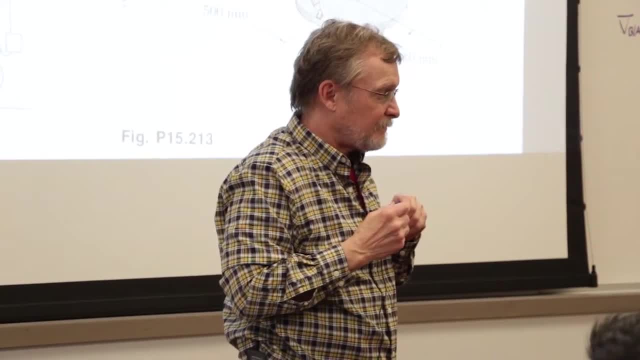 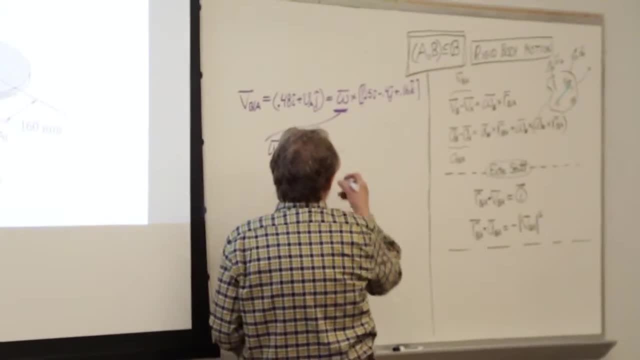 Would you agree that that's a complex rotation? Would you agree we don't know anything about that to start off with? That's a pretty complicated rotation. So to start off with, you'd have to say I don't know a thing about that vector. 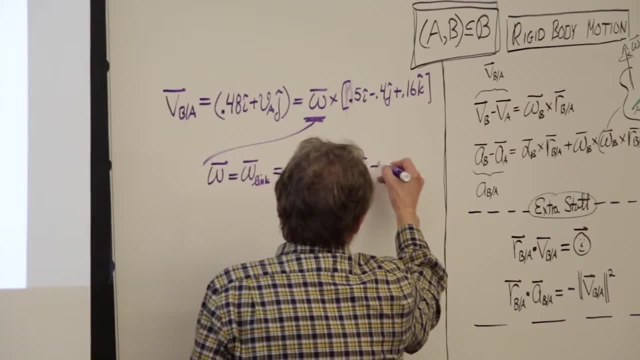 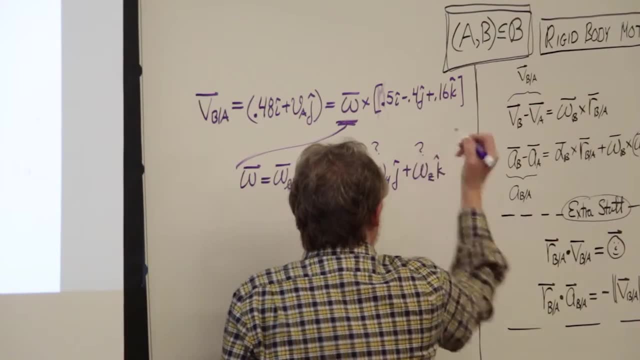 And if you're in a three-dimensional world with three-dimensional vectors, and if you have a vector you don't know anything about, then what you're really admitting, I think, is that you're talking about a vector which has three unknown components. 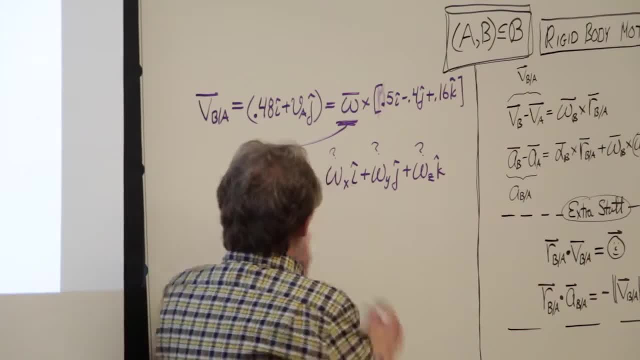 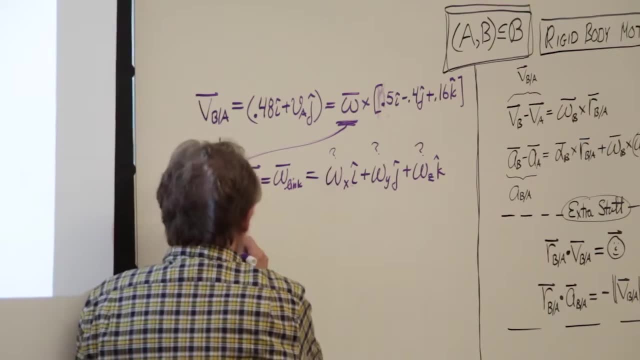 Yes, Okay now would you agree that he could put this expression in for omega? he could do the cross product- and would you agree that when he makes those substitutions, he could come up with three equations? He could come up with an I-component equation. 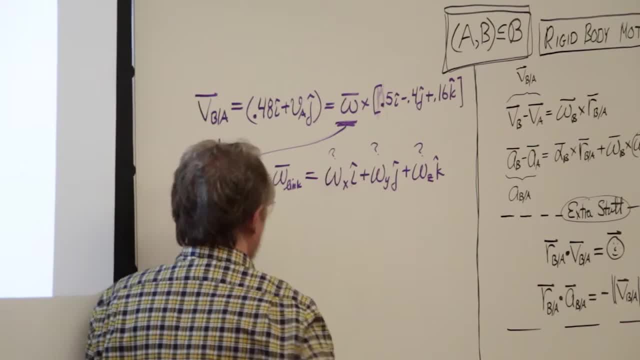 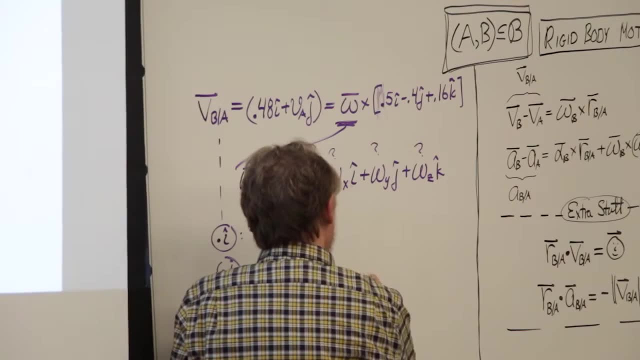 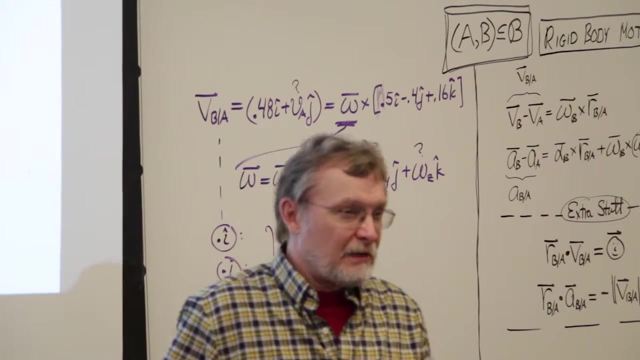 a J-component equation and a K-component equation And you would see three. I'll show you the Q's, I'll show you those in a moment. three equations. but how many unknowns would you see appearing in those three equations? 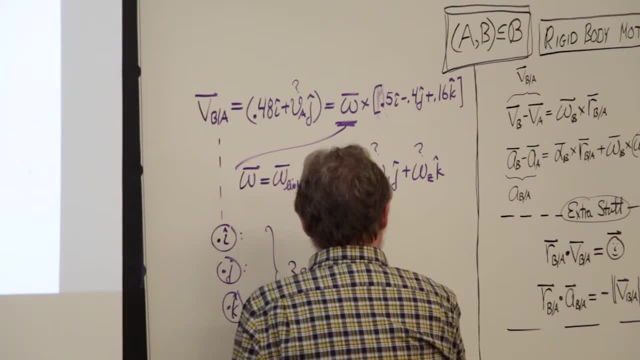 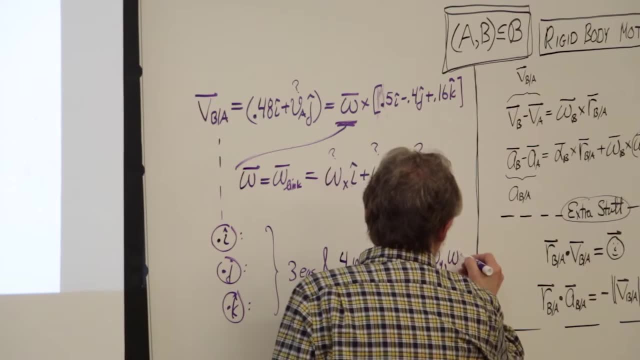 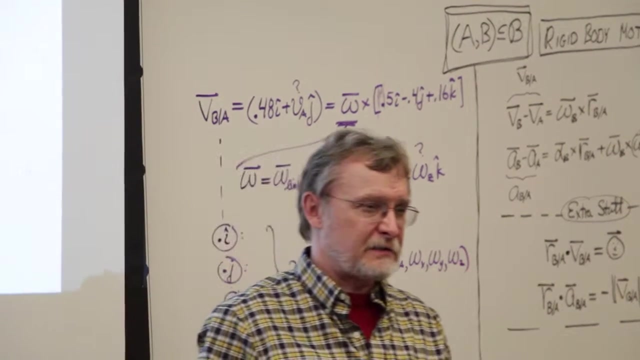 There'd be four unknowns, And the four unknowns would be VA, omega sub X, omega sub Y and omega sub Z, and the last time I checked, you generally can't solve for four unknowns if you only have three equations. 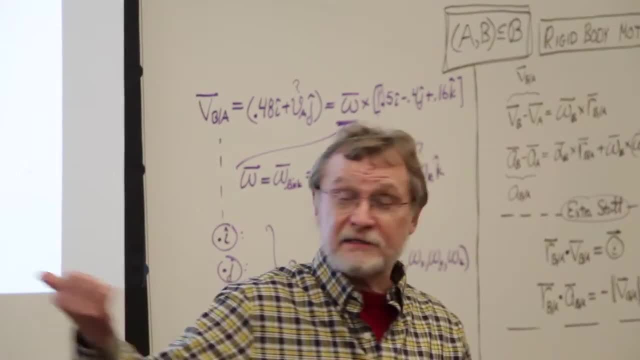 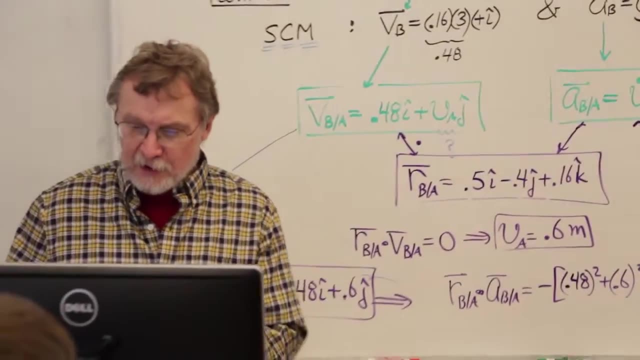 So what did he do to get around that? Because he did get the solution. He got the same solution that I did, at least for part A. He didn't even attempt part B, okay, But he got the same solution. Now, how did he do it? 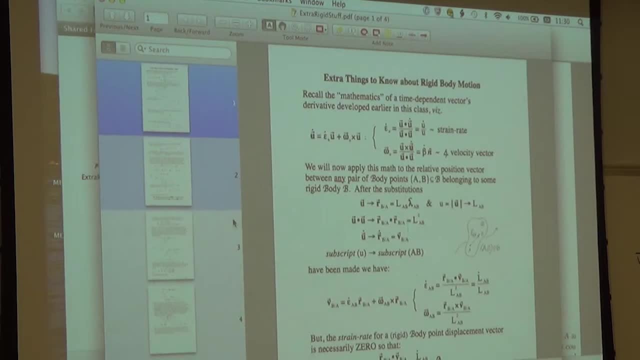 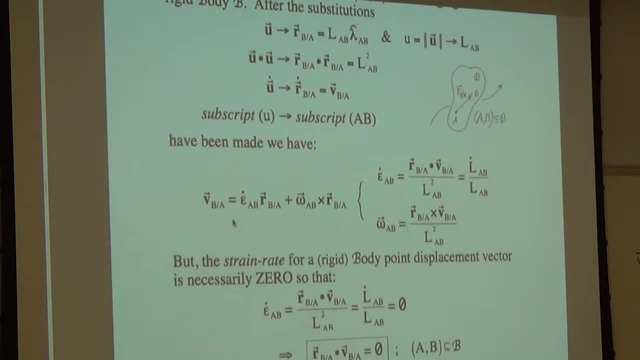 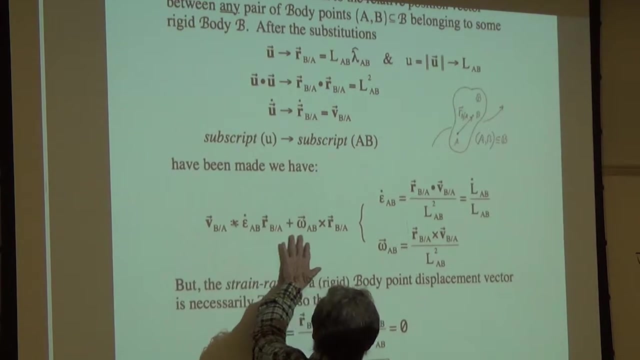 How did he get around that difficulty? Well, let's go back to that extra stuff handout, because there's more to it. Once we figured out, or once we made the observation, remember we had using the mathematics from week two. 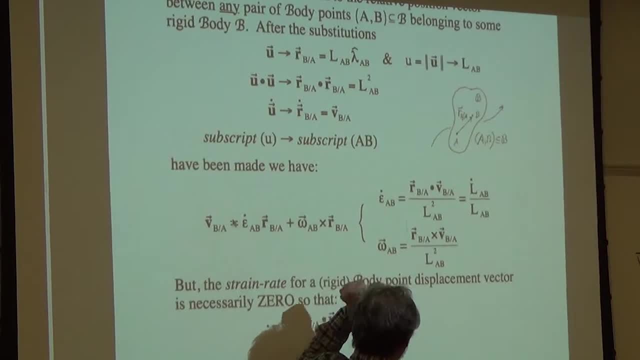 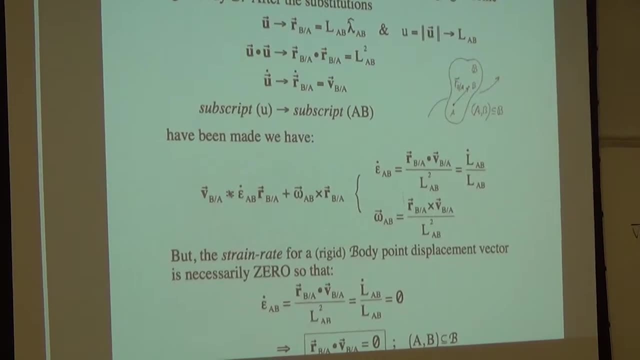 we came up with this expression in terms of strain rate and angular velocity, and once we figured out that the strain rate was equal to zero, had to be equal to zero, leading us to this and then to this equation. we could have gone back to this equation. 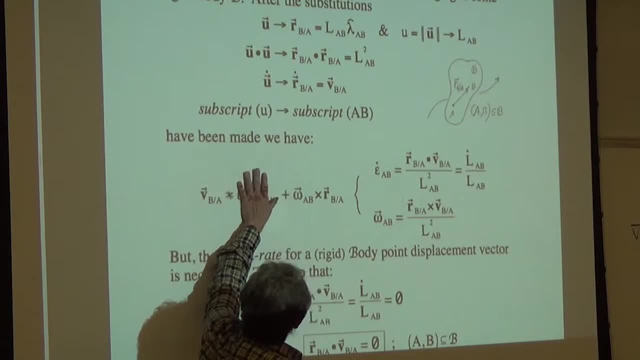 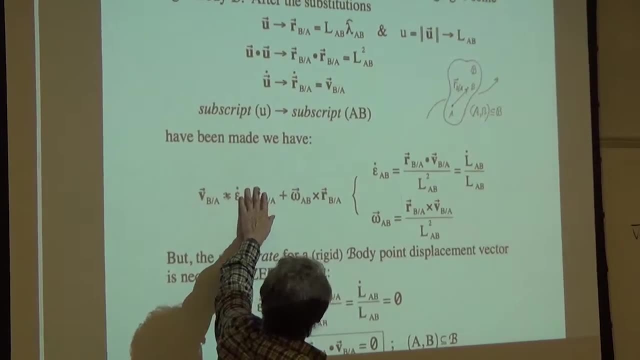 to see what was left of it. If you set epsilon dot equal to zero, then that term goes away, and since we have the equation over there, I guess you can just erase that completely. so what you're left with is VB slash A. 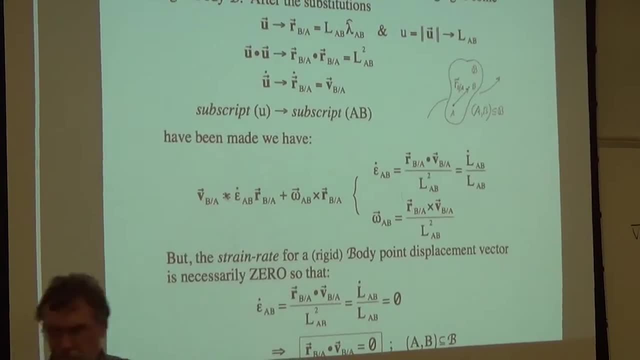 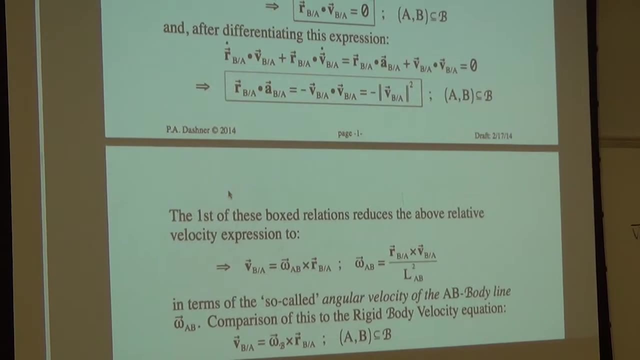 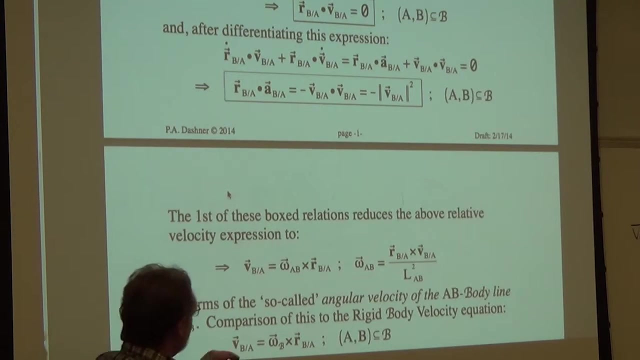 equal to this vector crossed with R. So we move on to page two of these notes, Getting rid of the strain rate as we have. what's left reduces to that which says that the relative velocity of the two body points A and B is equal to the angular. 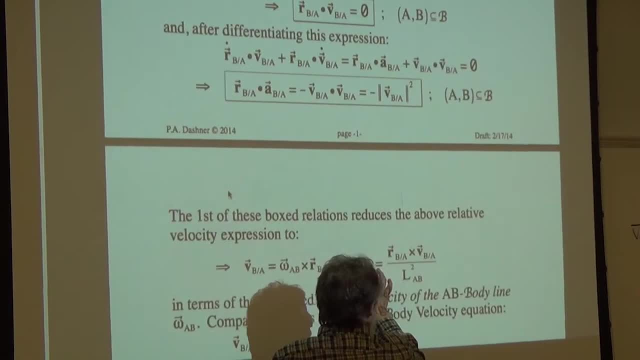 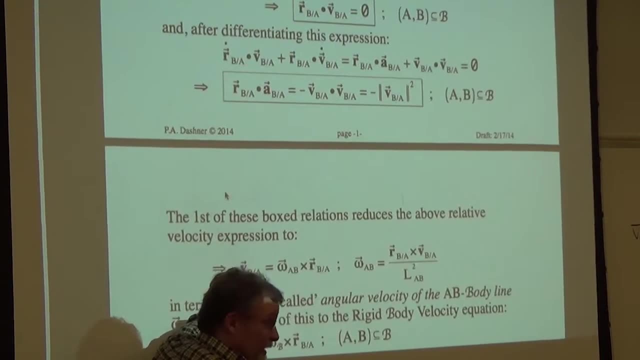 what do we call this? We call this the angular velocity of the AB body line. That's what that's called: the angular velocity of the AB body line. We learned that the relative velocity is equal to the angular velocity of the AB body line. 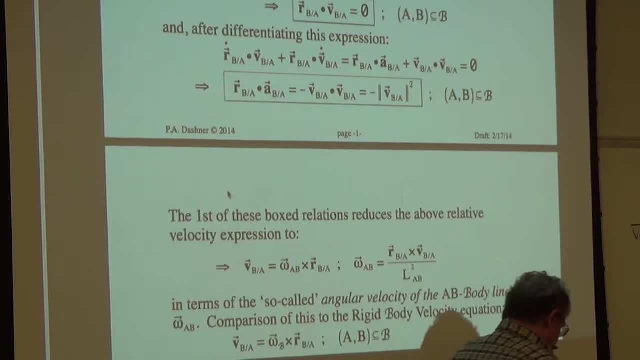 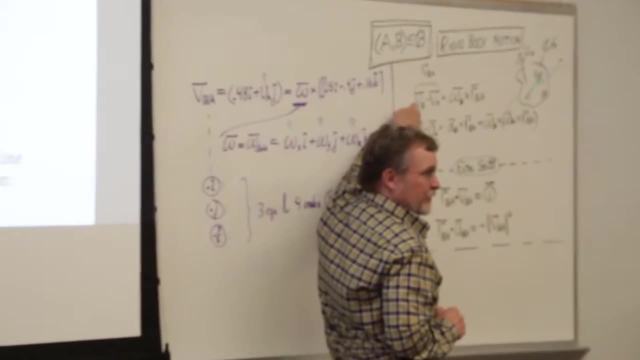 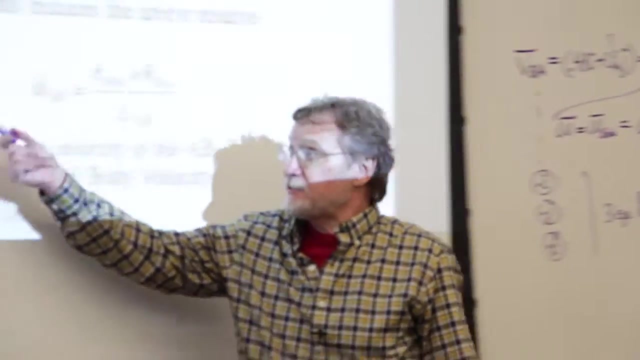 crossed with the relative position vector. But gee, doesn't that equation look stunningly like this equation? This equation is expressed in terms of the unique angular velocity of the body, whereas this equation is. the omega in this equation is given by a specific formula. 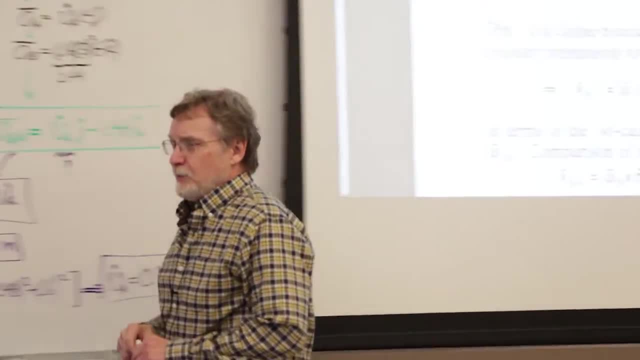 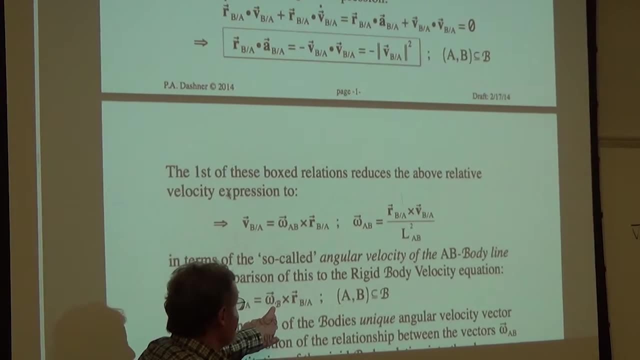 and it's called the angular velocity of the AB body line. But both equations are true. Both equations are true. This equation is true in terms of the body's unique angular velocity vector. It's one and only one angular velocity vector, and this equation is also. 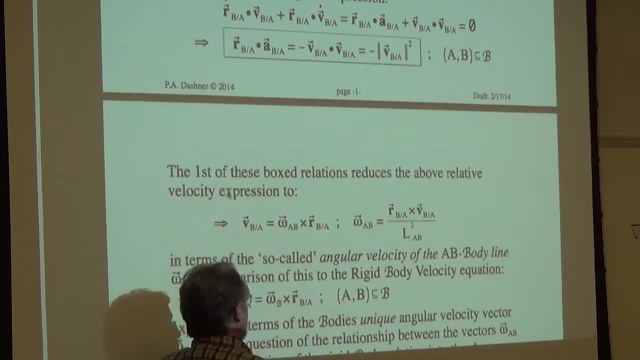 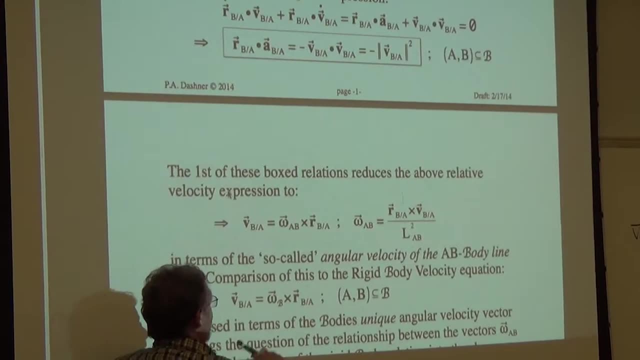 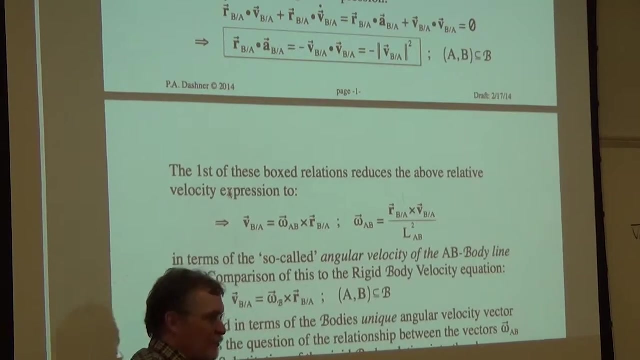 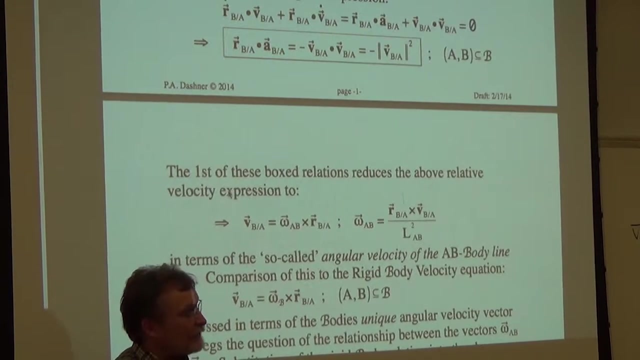 true, but expressed in terms of the angular velocity of the A-B body line. And then the question comes up immediately is: since both of these equations are true, does that imply a relationship between the angular velocity of the body and the angular velocity of the A-B body line, For instance? does it say that they are equal? They could be, but most 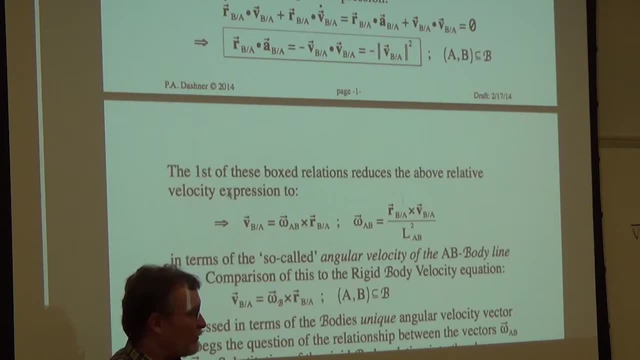 of the time they're not. They could be equal, but most of the time they're not. So let me just show you how much different those two vectors can be. And how is it that, even if they are different, how is it that both equations could be true? Well, I'll establish that in. 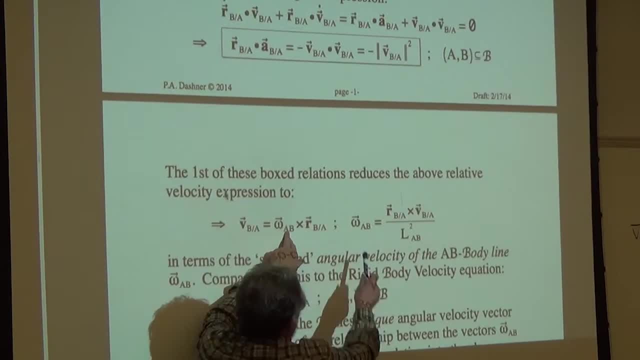 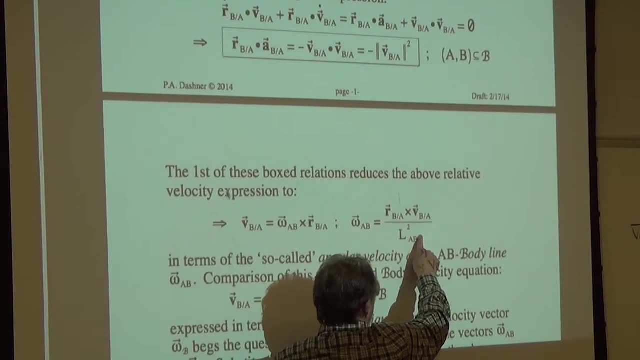 just a moment. What I'm going to do to show you the relationship between this vector and the body's unique angular velocity vector is: I'm going to take this equation for the angular velocity of the A-B body line and I'm going to make a substitution. I'm going 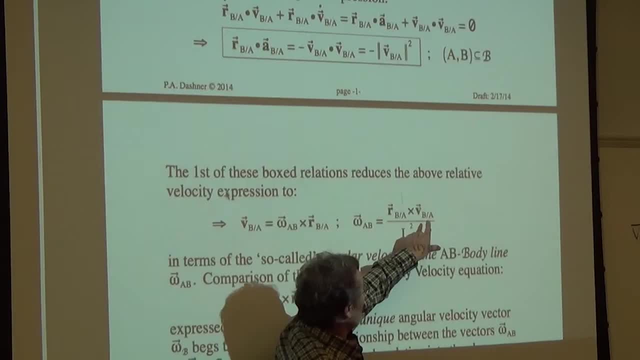 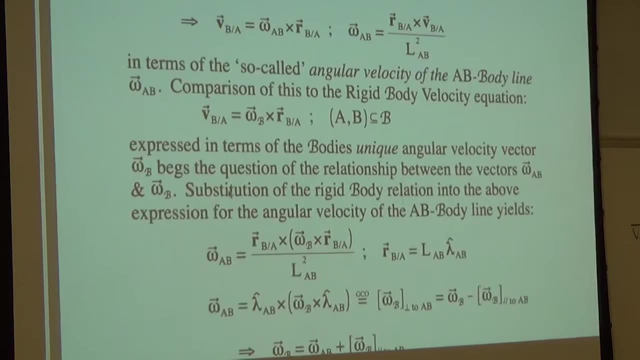 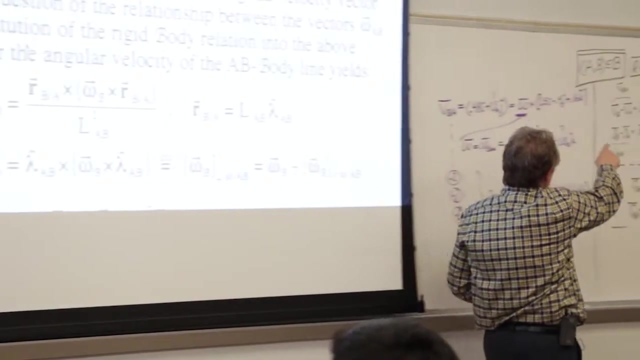 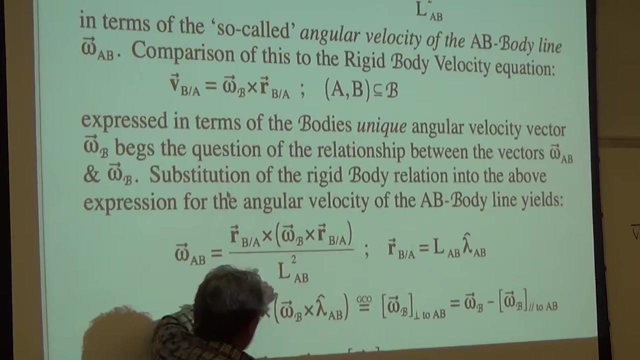 to make this substitution right there, And when I do- and you can do this on your own time- you end up with the following: Let's blow it up real big. When you make the this A-B body line angular velocity expression, you get this, But remember the position vector. 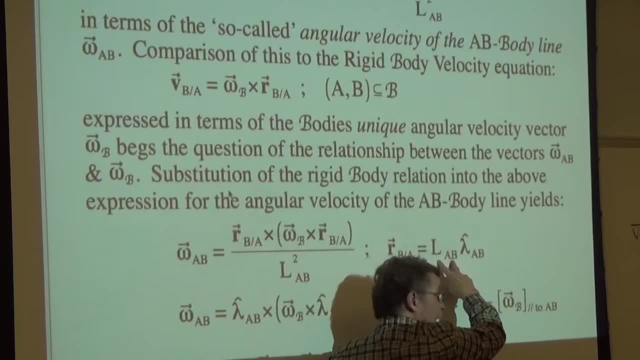 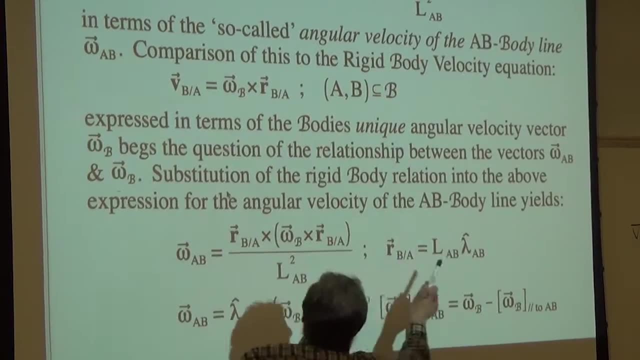 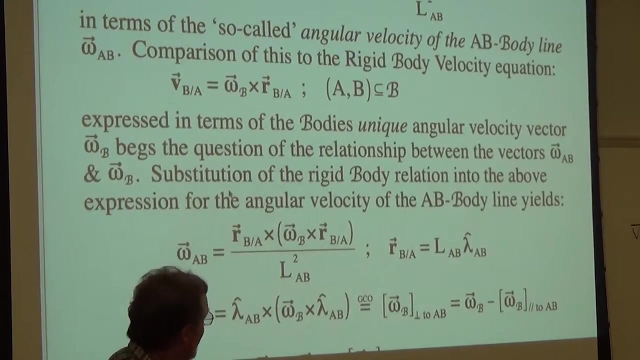 the relative position vector is a vector with a magnitude equal to the length of that line times the unit vector pointing in that direction. What happens if you make this substitution for R in both spots? What happens to the capital L's? They all cancel out and you're left with 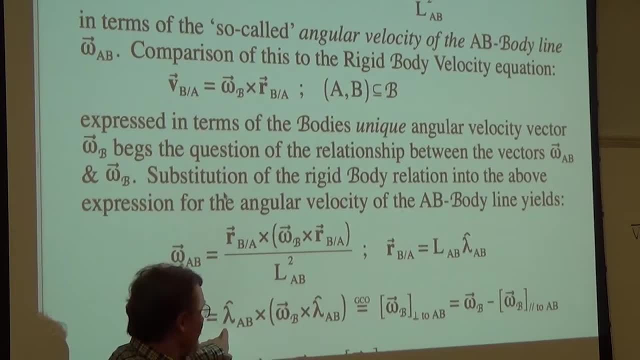 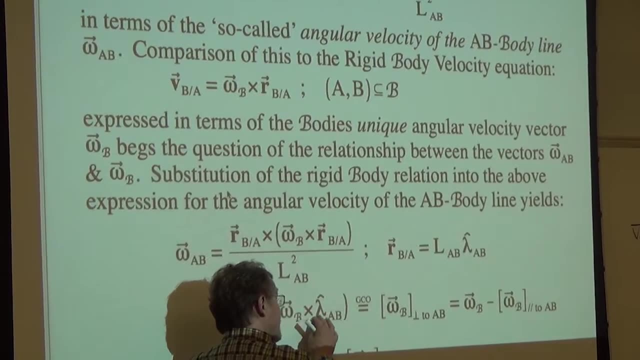 this And I hope you don't have to actually go back to page one of the general course. This outline, But do you recognize unit vector crossed with a vector crossed with a unit vector? Do you? does that form appear near the top of page one of the general course? 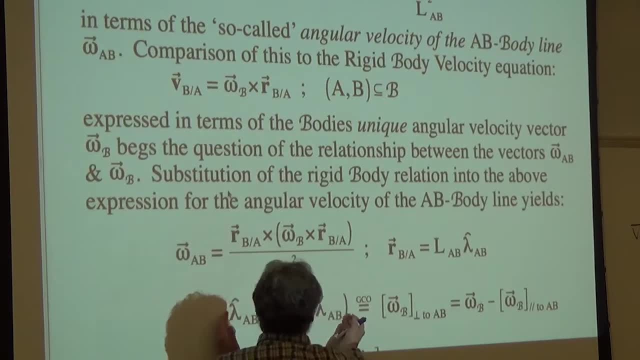 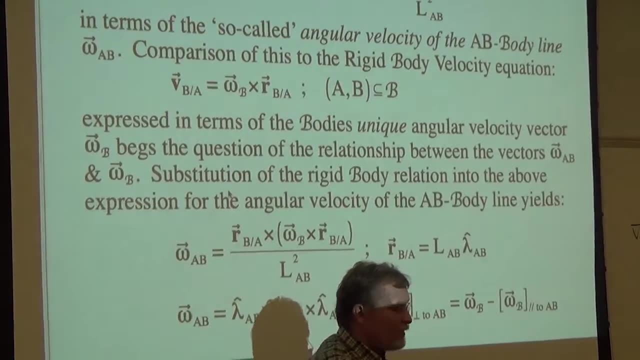 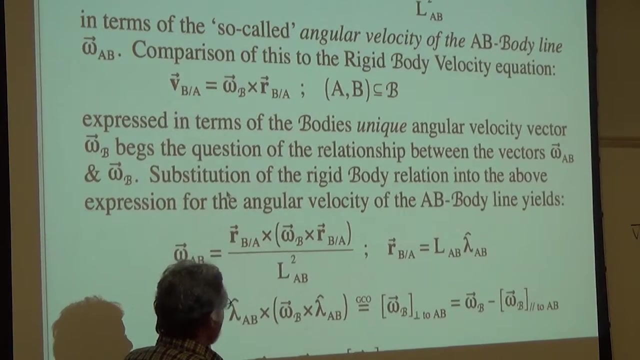 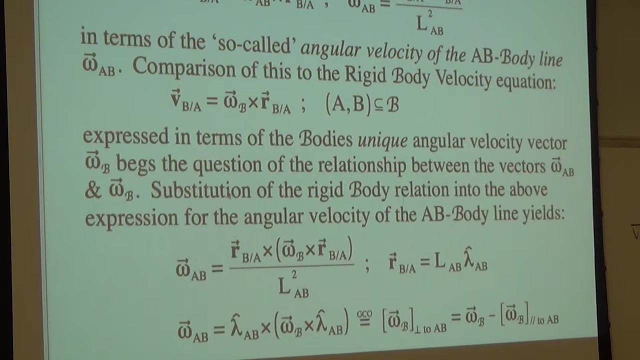 outline. Is that not the specific formula for computing the rectangular component of this vector, which is perpendicular to A-B? So what we've established is that the angular velocity of the A-B body line, given by the equation right at the top of the screen, the angular velocity of the A-B body line is in: 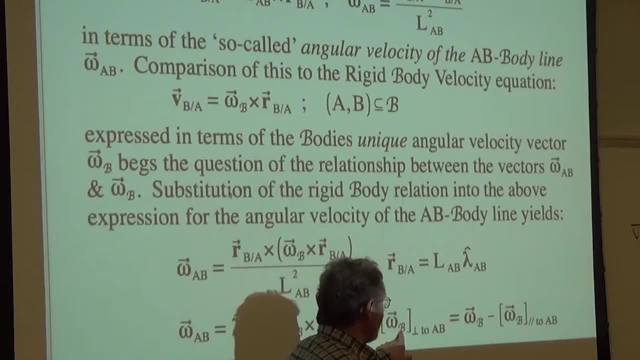 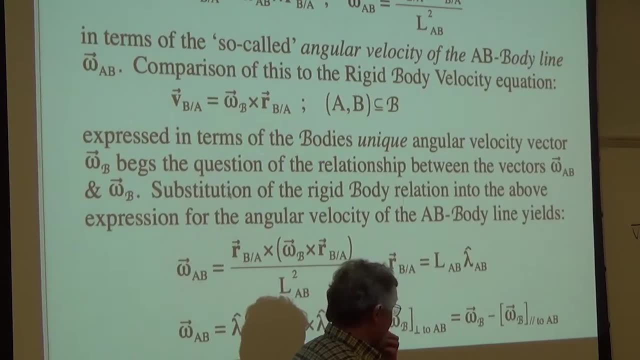 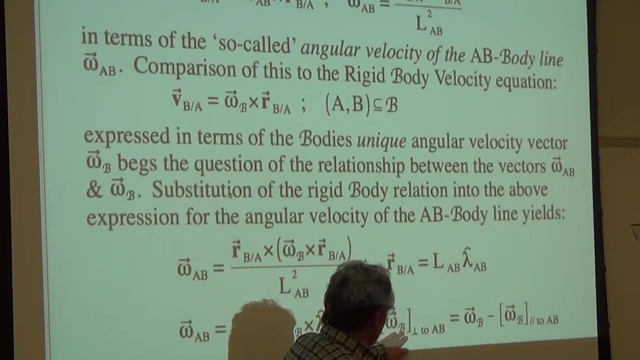 fact equal to the portion of the body's angular velocity vector which is perpendicular to A-B. It's kind of cool. In other words, they don't necessarily have to be the same, apparently. By the way, would you agree that the angular velocity of the body could be exposed to a? 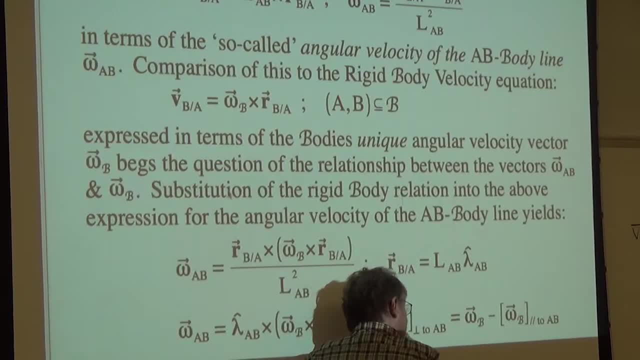 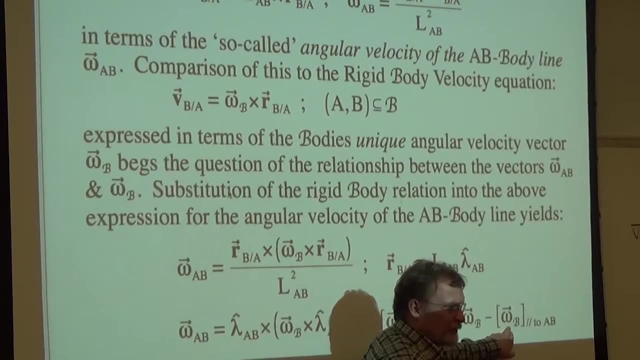 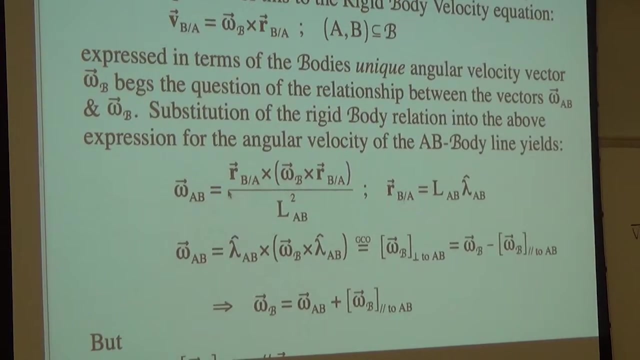 parallel perpendicular deconversion. In fact, would you agree that the portion of omega of the body which is perpendicular to A-B would be the entire vector, minus whatever portion was parallel to it? Would you further agree that? well, I guess let's turn that around a little bit, Let's actually take that. 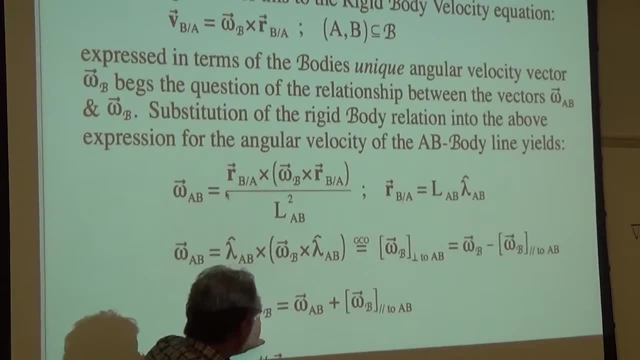 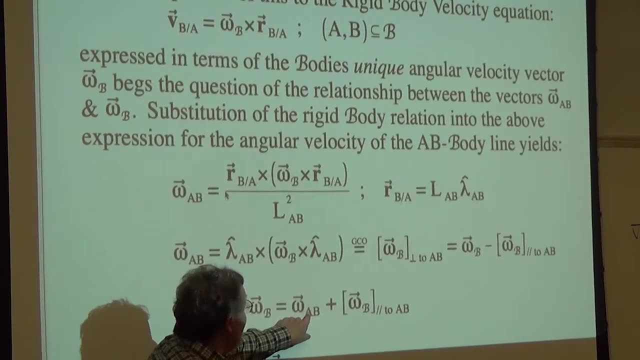 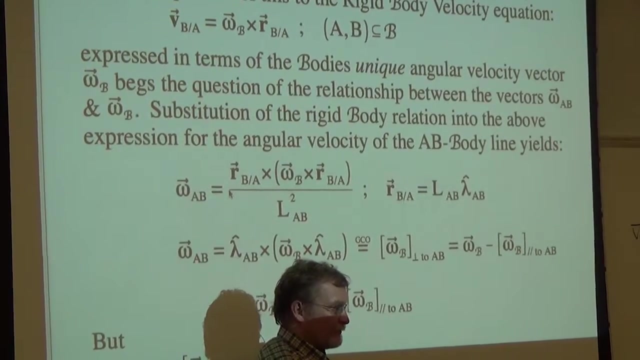 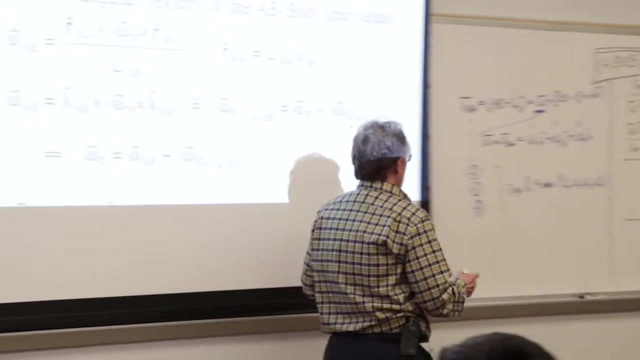 expression right there and say: therefore, the body's unique angular velocity vector is equal to the angular velocity of the A-B body line. Okay, Plus whatever component it would have which is parallel to A-B. By the way, what we've really established- I mean, let me highlight that over here- We've established that the 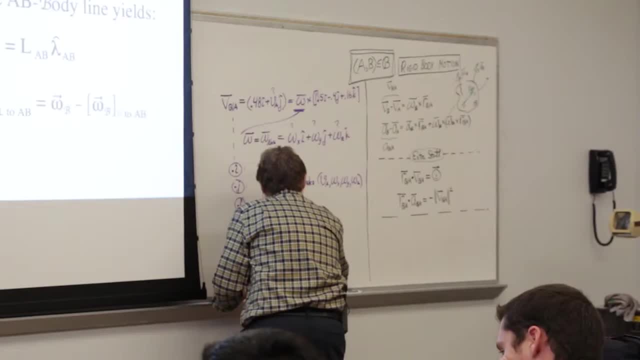 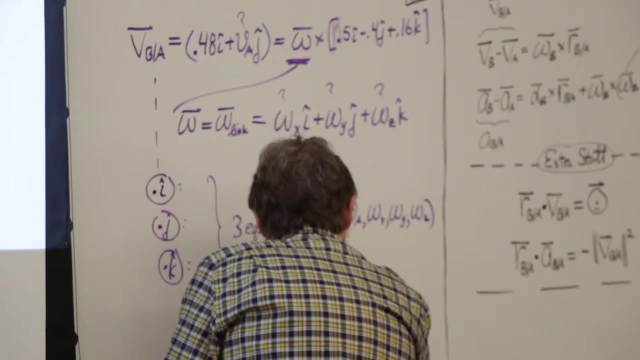 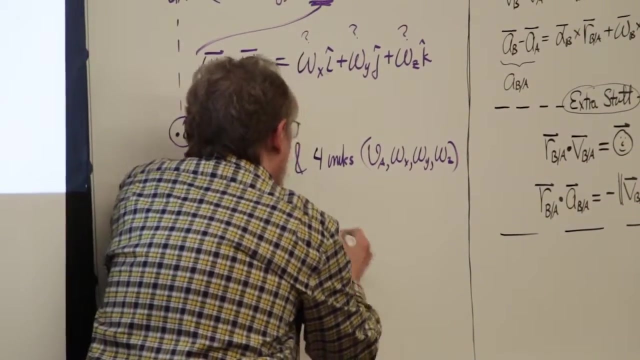 angular velocity of the A-B body line, as given by that specific equation, is equal to the angular velocity of the body which is perpendicular to the A-B body line. And, by the way, a little notation. So guess what? Miriam and Craig give this part of the angular velocity, vector a. 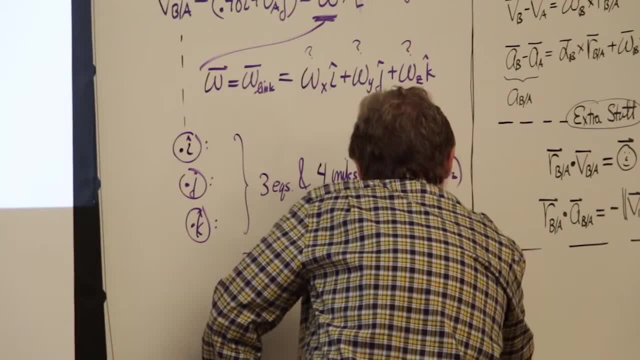 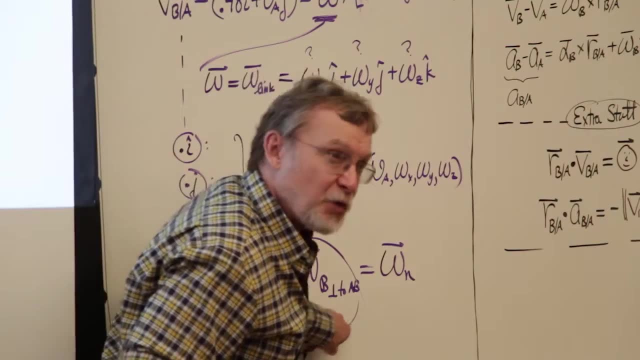 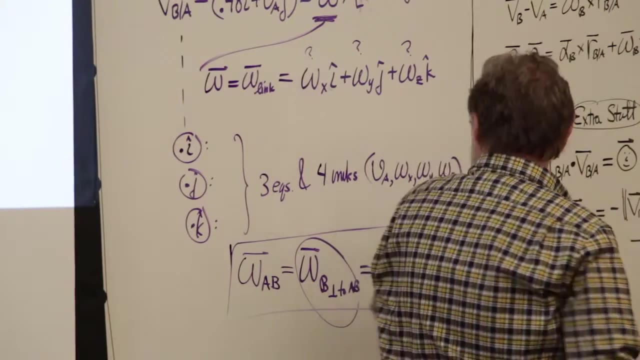 special name. They call it omega sub n. They call it omega sub n when you look at their problem solutions: N for normal or perpendicular, N for normal to or perpendicular to the line. So they call that part of the body's angular velocity vector. they call it omega sub n. 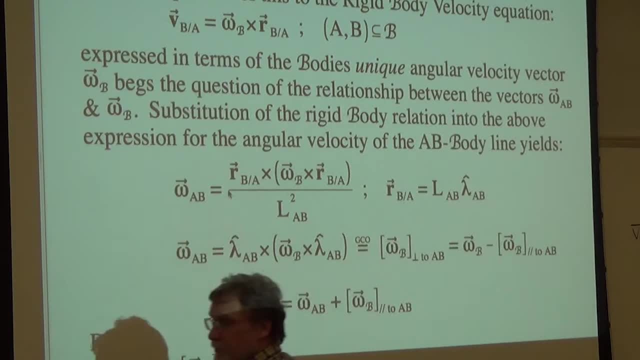 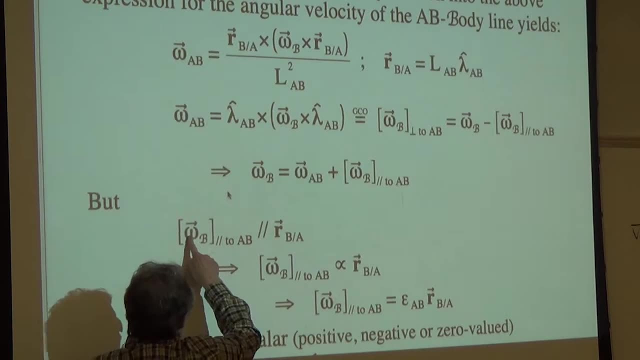 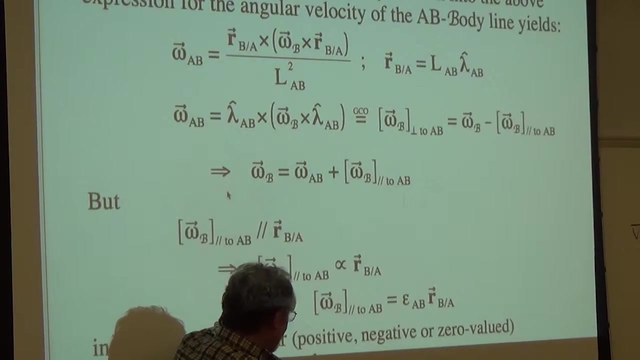 the normal part of it. Okay, Well, let's continue on to the bottom of the page. Would you agree that if the body's omega vector had a component which is parallel to AB, then would you agree that that portion of the omega vector would be proportional to that vector? 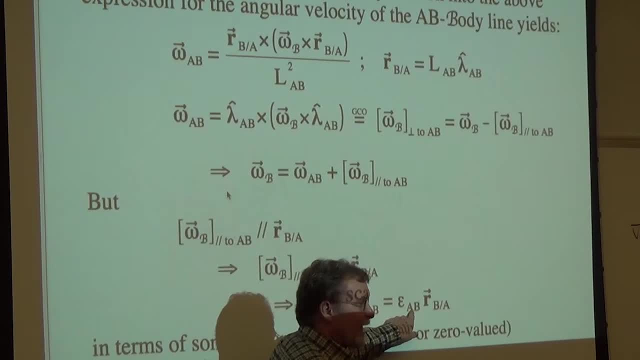 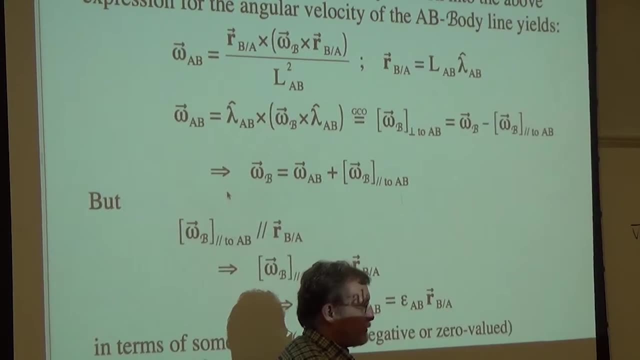 And if two vectors are proportional, would you agree? there would have to be some scalar value of proportionality that would fit into this equation. If two vectors are proportional to one another, there must be some constant proportionality, And I'll give it the name epsilon AB. 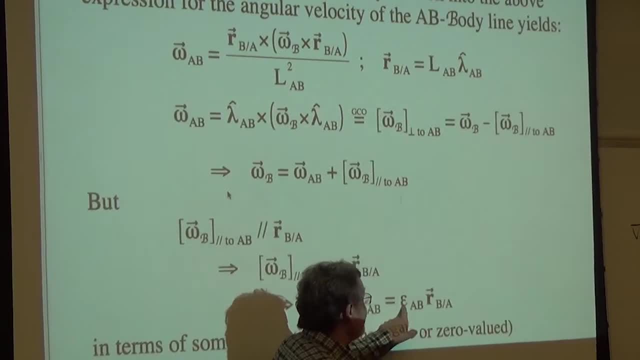 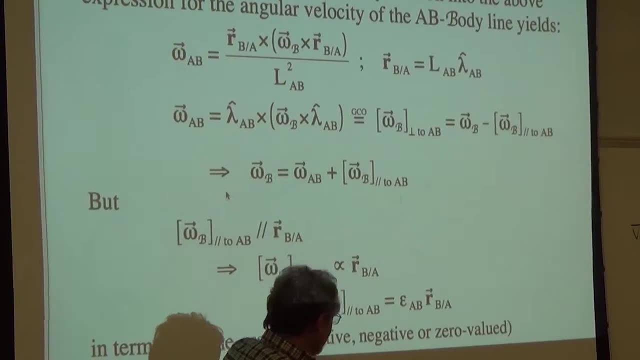 It's not a strain rate, It's just some number. It's some either positive, negative or maybe even zero valued number. We're just saying that this part of the body's omega vector is expressible as a multiple, a scalar multiple, of that relative position vector. 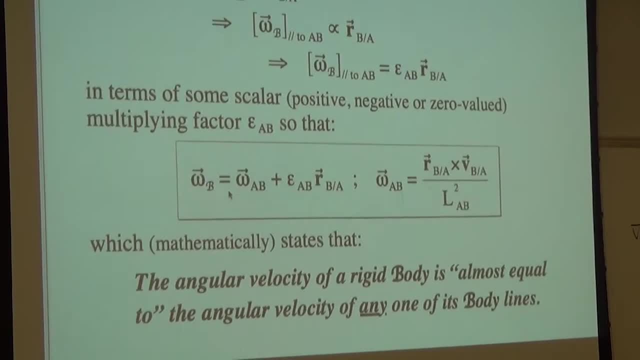 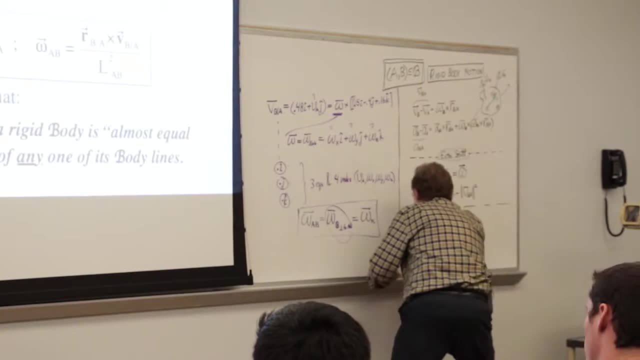 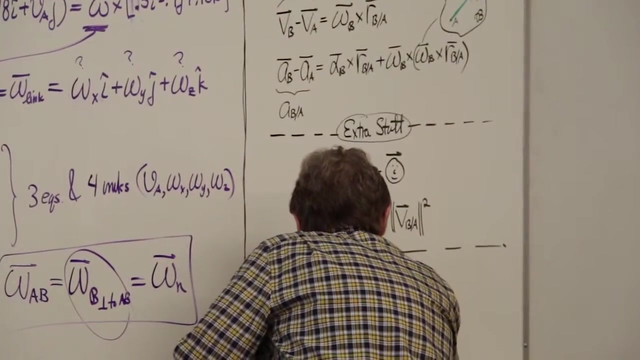 And that leads to this equation in the box and the statement that goes with it, which is the sort of the last extra thing we need to know about rigid body motion. This equation says That the angular velocity of a body is equal to the angular velocity of any one of its 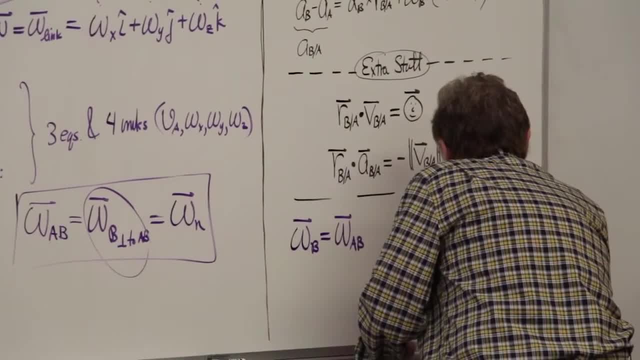 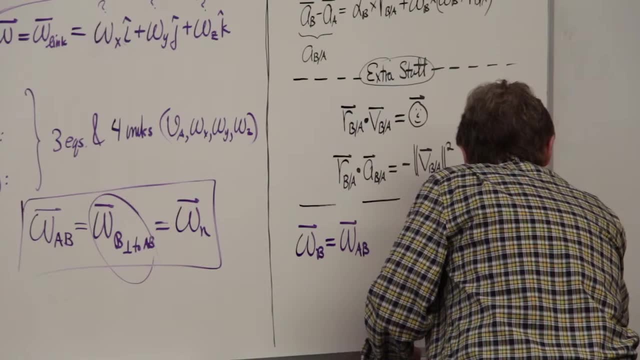 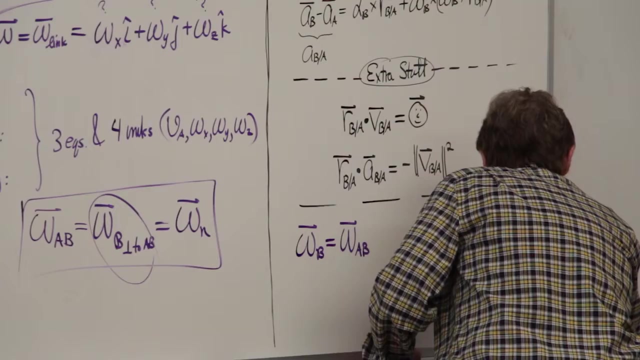 lines as given by a specific formula. The angular velocity of the AB body line is the relative position vector between those two points crossed with the relative velocity vector for those two points divided by the square of the distance between those two points. That is the definition of what's called the angular 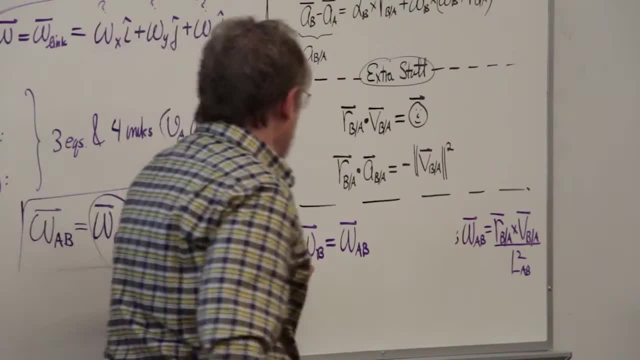 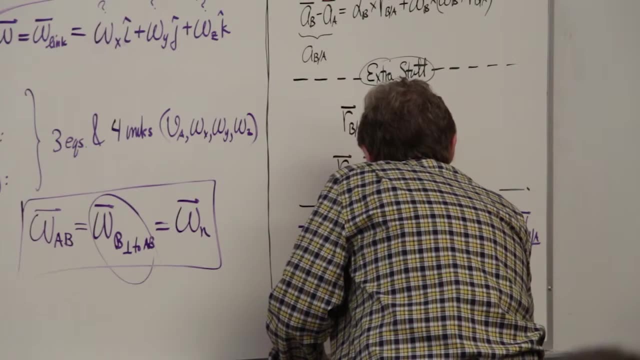 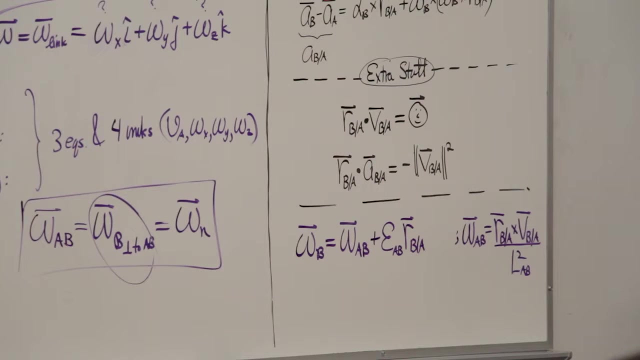 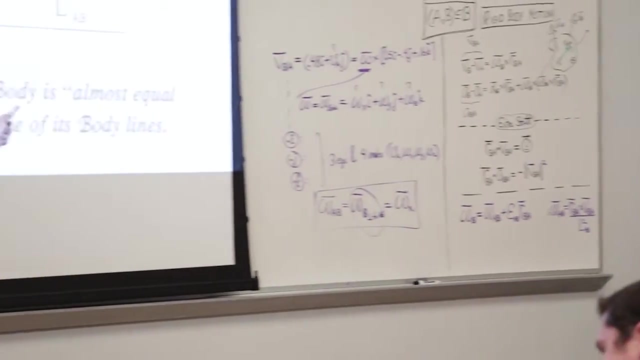 Angular Angular velocity of the AB body line And the angular velocity of the body is equal to that, plus perhaps some extra scalar multiplier multiplying the relative position vector. That's the last extra fact that I want you to be aware of, And the words that I put with that equation are that the angular velocity of a rigid body 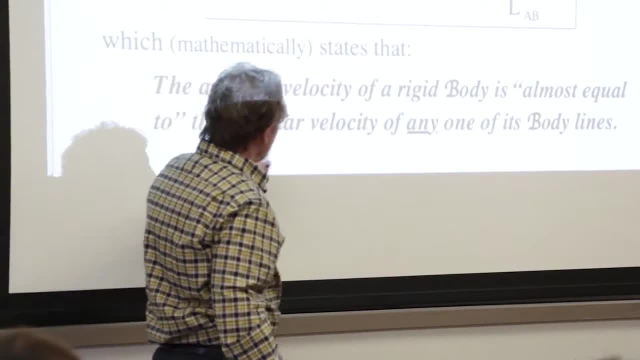 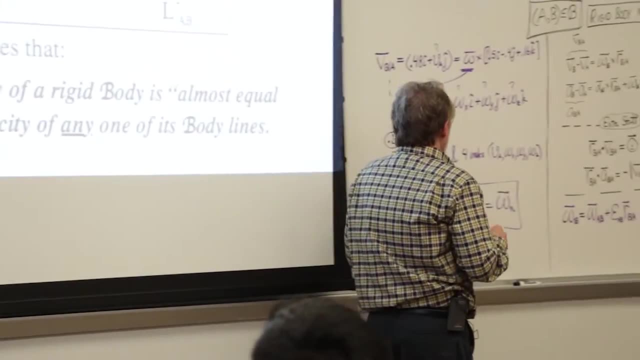 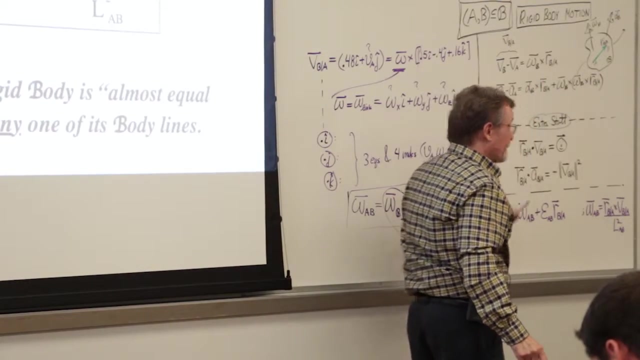 is- quote- almost equal to the angular velocity of AB, The angular velocity of any one of its body lines. Let me justify those words. If you have a body experiencing three-dimensional motion, then you know it has an. it does have a unique angular velocity vector. 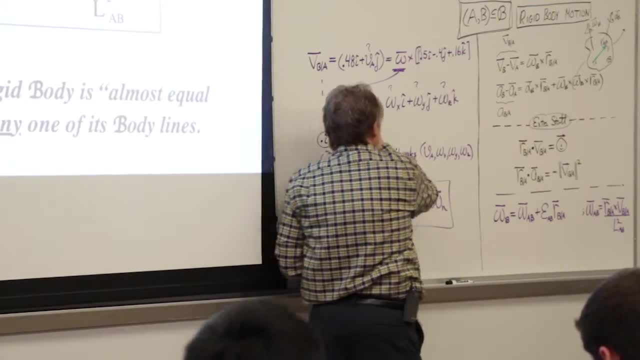 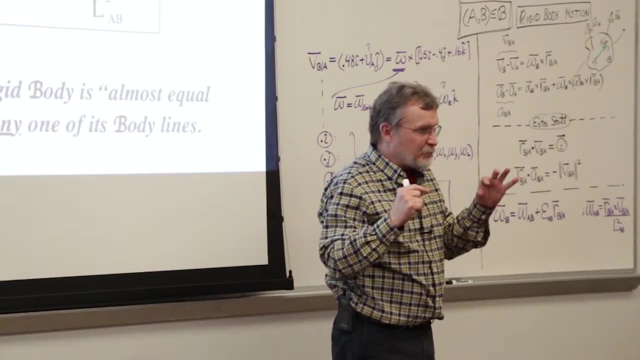 But I can. the problem we're doing with the link. would you agree that we don't know squat about the angular velocity vector of the link? And again, if you, if a three-dimensional vector is completely unknown, you're at a level of three as far as unknowns are concerned. 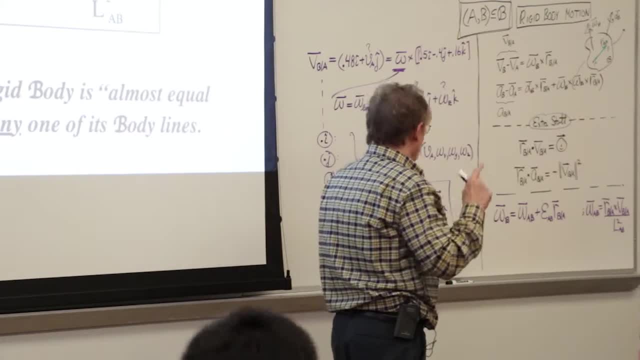 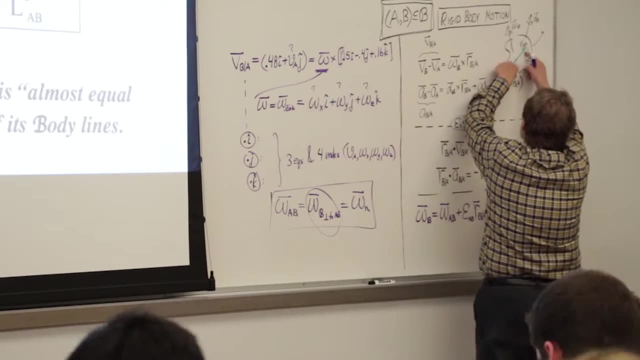 There's three things that are not known. There's three things that are not known, But suppose. suppose you were able to figure out the velocities of two points in the body. Suppose you can find two points in the body for which you know the velocity. 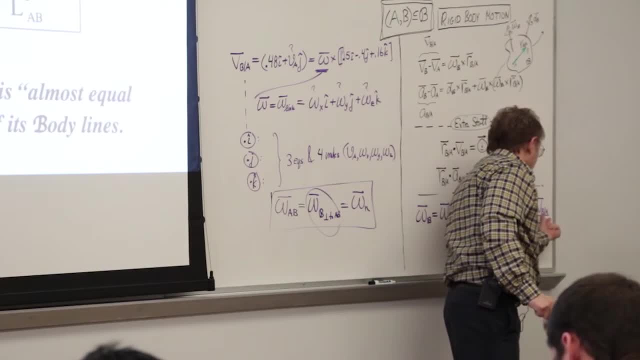 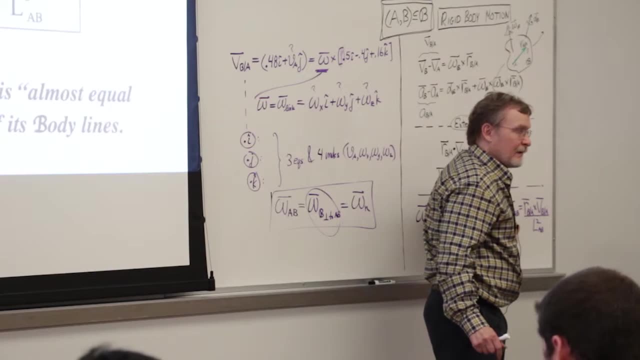 Would you agree that if you can find the velocities of two points in the body, you could compute the relative velocity, And by this formula you could, you could compute the angular velocity of that body line? Okay, Then how far along the road to finding this would you be? 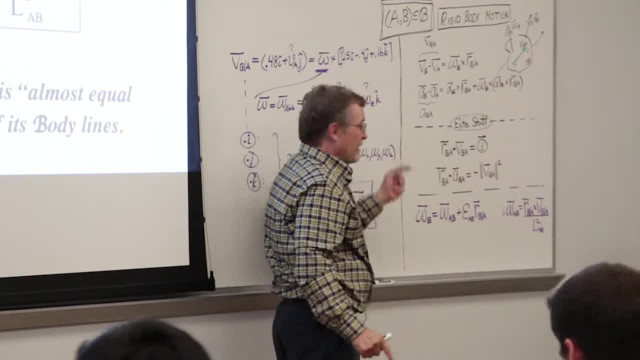 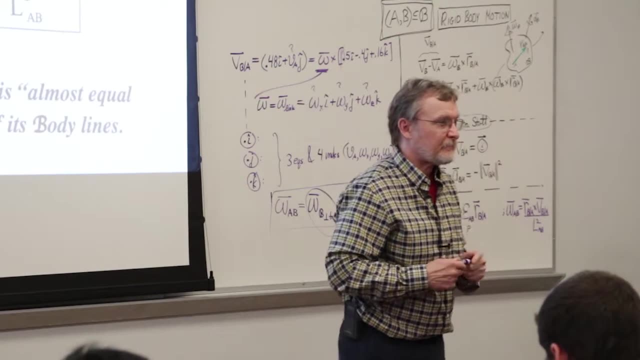 You know you started off not knowing anything about that vector right, Three unknowns. You would have reduced the problem of three unknowns to one unknown. So if you can ever figure out the velocities of two points in a body, you're two-thirds. 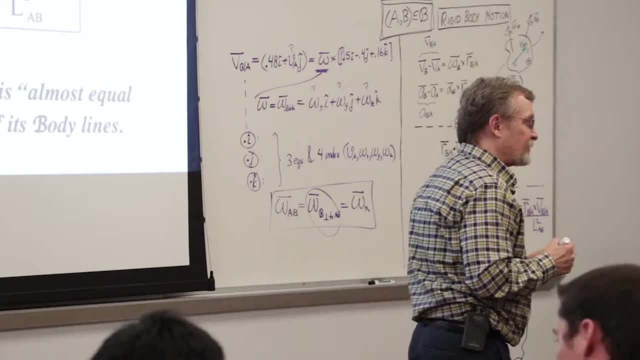 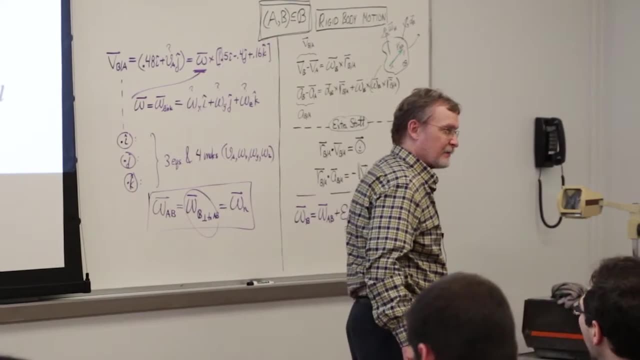 of the way to knowing what the angular velocity actually is. Now there's another reason why you know you've never seen this equation before, because it doesn't come up in two-dimensional dynamics. But I can convince you that there has to be. 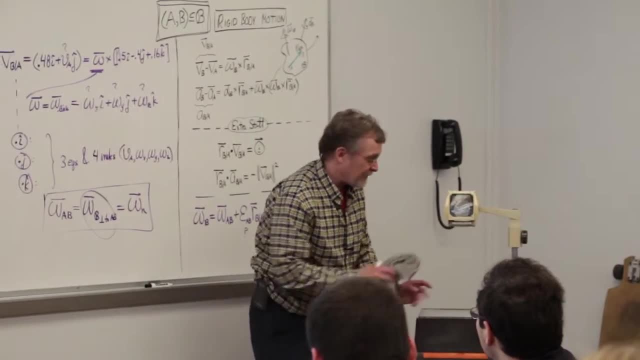 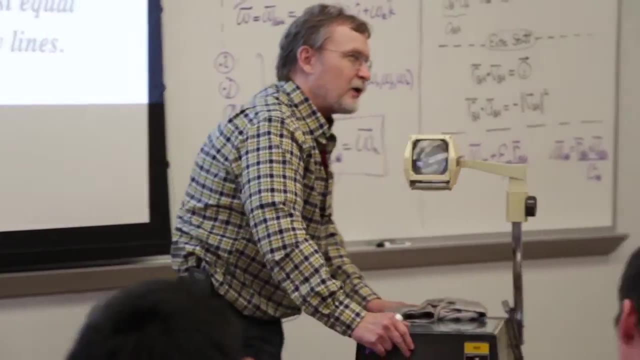 Okay, There has to be an equation like that, Because here's essentially a rigid body. Would you agree that this rigid body is undergoing what you'd call planar motion, And would you agree that right now, what? what can you visualize its angular velocity? 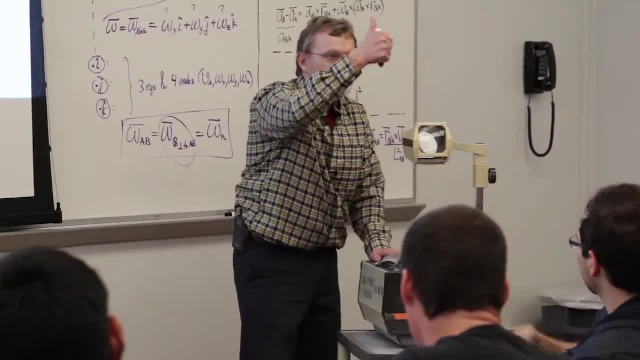 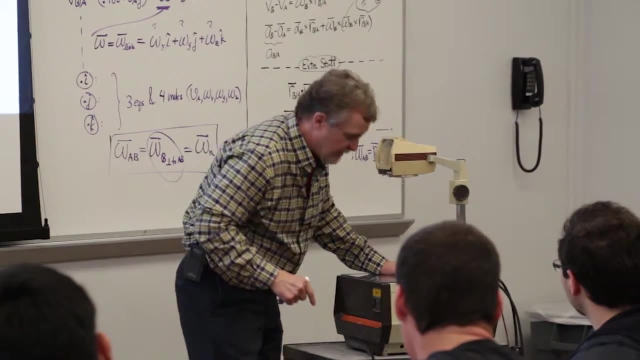 vector right now Points in what direction? Straight up in this direction. Okay, Well, there has to be an equation, something like this, and I'll tell you why. Notice, I've marked two body points. Now the side of this is a little bit slow. 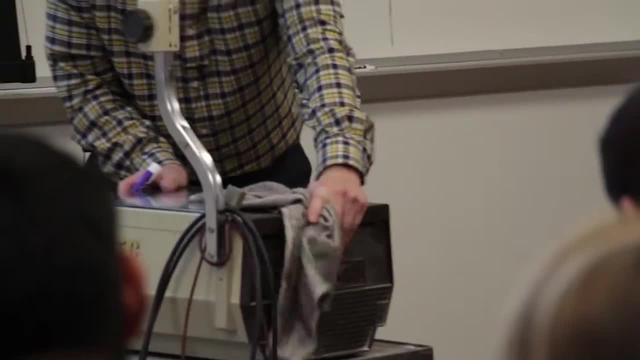 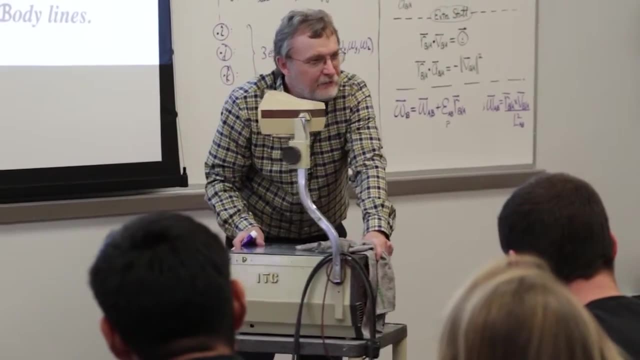 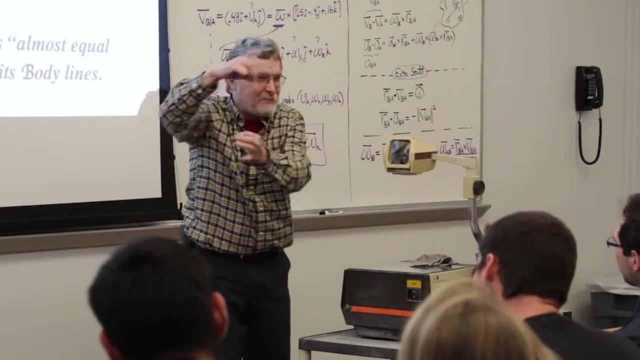 Let's assume that it's vertical. Are those two points moving? Tell me something about their velocity vectors? Not just parallel? They're exactly the same. The points are right above and below one another, So they have exactly the same motion. They're both moving with planar motion. 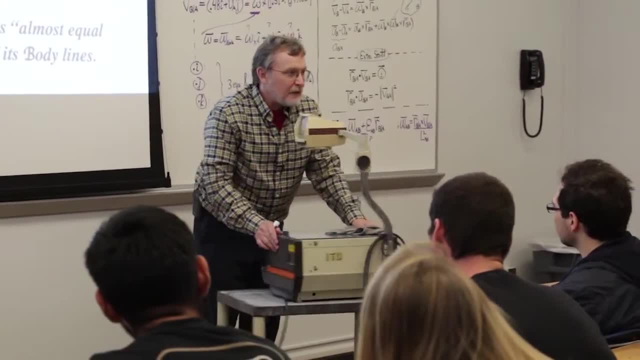 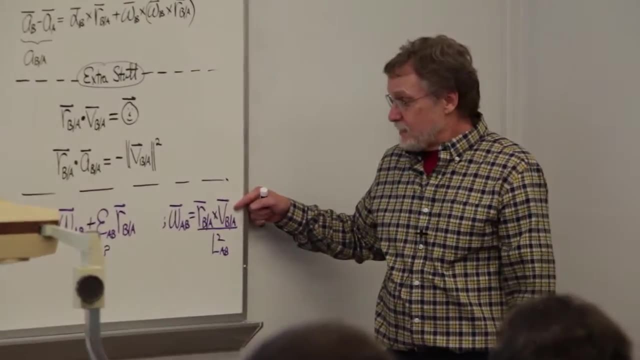 The velocity vector is absolutely identical. The velocity of A is equal to the velocity of B. Okay, So therefore, what's the relative velocity? Zero Zero. So what's the angular velocity of that AB body line? Zero, Zero. So what does this equation say? 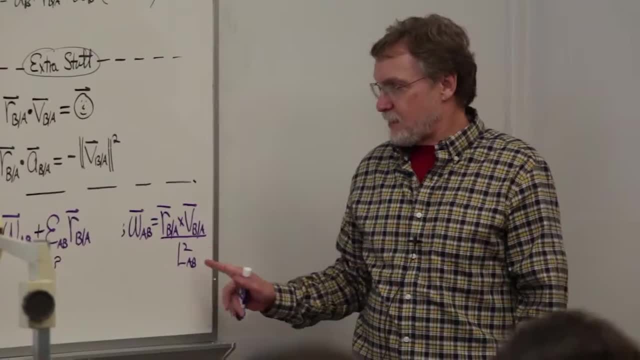 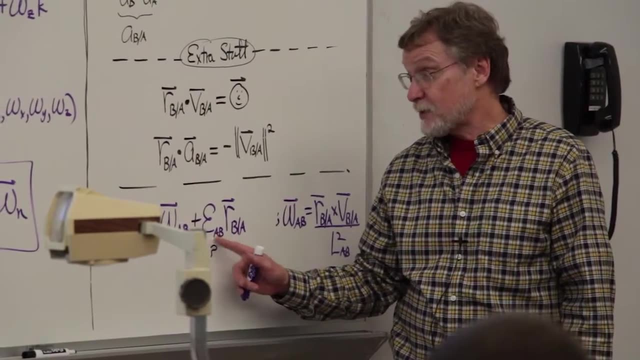 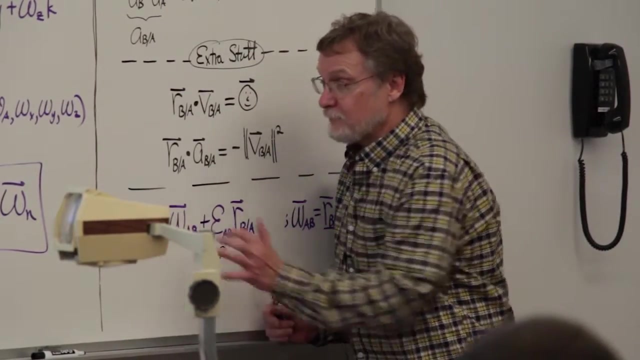 It says that the angular velocity of that body is equal to zero, plus perhaps something in the direction of that line. If this term wasn't there, if you thought that the angular velocity of a body was equal to the angular velocity of any one of its lines, you'd be screwed. 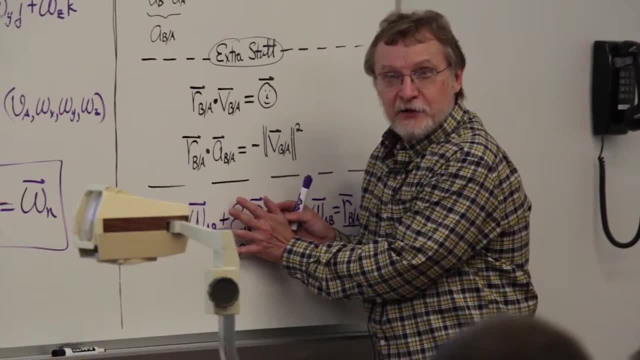 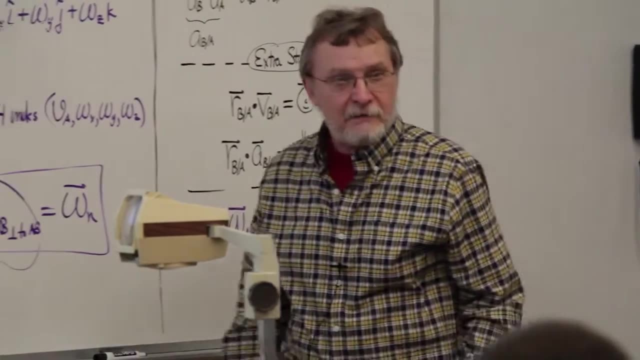 If this term wasn't there, you'd be stuck with having to say: oh, because this is zero, the body's not rotating. Well, it's just not so. Now, that issue doesn't come up in two-dimensional analysis, but it obviously comes up in three-dimensional. 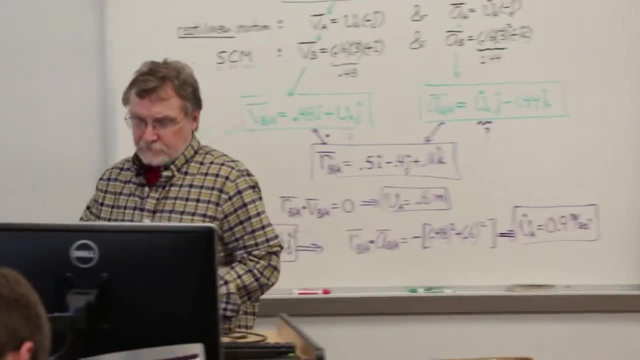 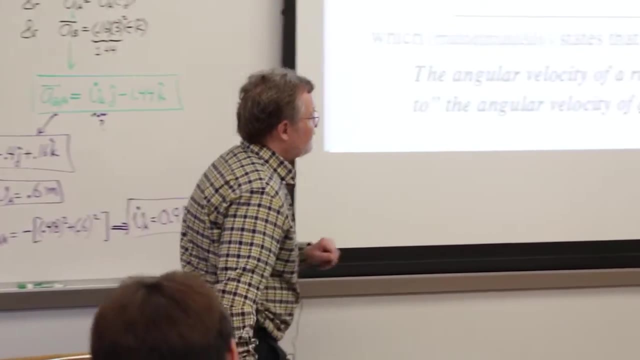 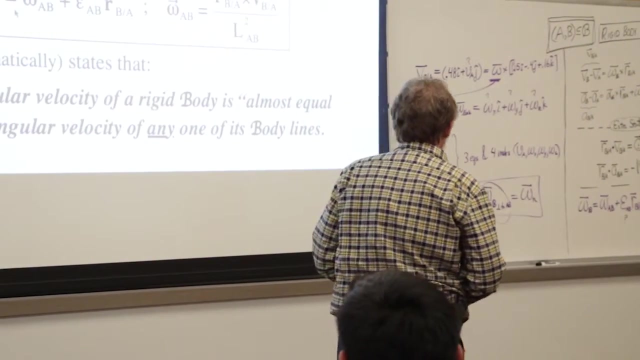 analysis, and it's extremely important. Okay, Now let me, oh, let's show you how Beer and Johnson used that fact to actually finesse the problem that I mentioned of the three-equation: Four equations and four unknowns. What he realized was the following: 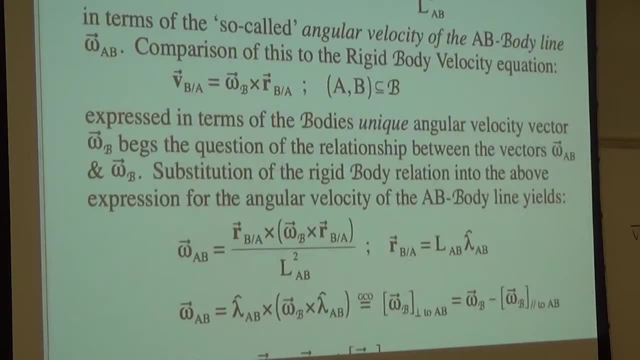 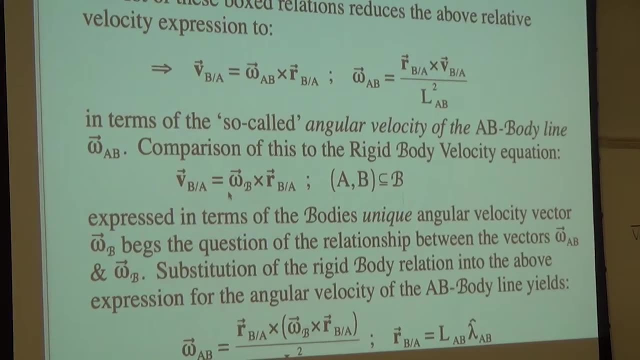 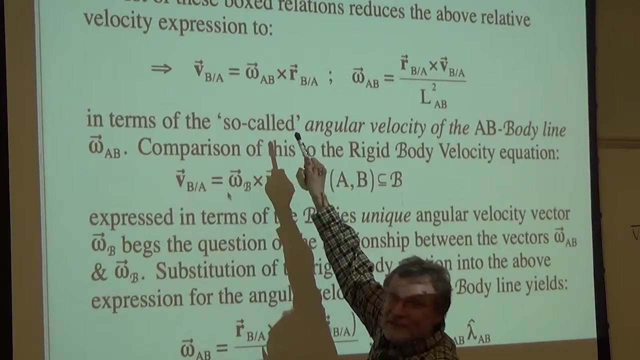 What he realized was that, as far as the relative velocity equation between any two specified points, as far as this equation is concerned, you don't need to have the full angular velocity in there. You don't need it. All you need is that. 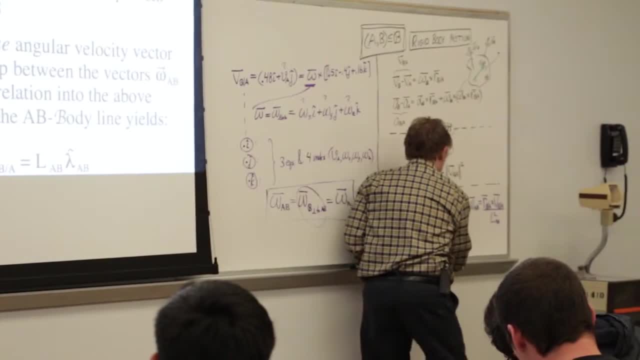 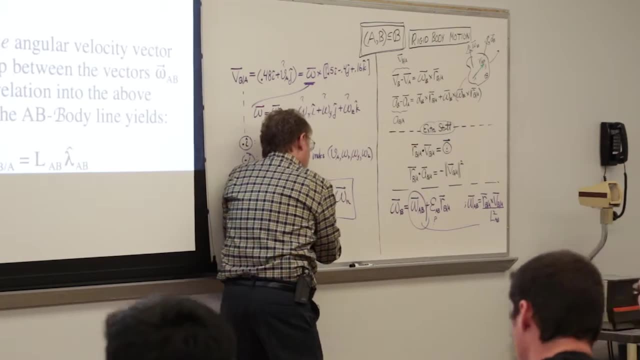 All you need is this part right here. All you need is this part And this part, as I've already pointed out to you, the angular velocity of the AB body line is the portion of the body's angular velocity which is perpendicular to AB. 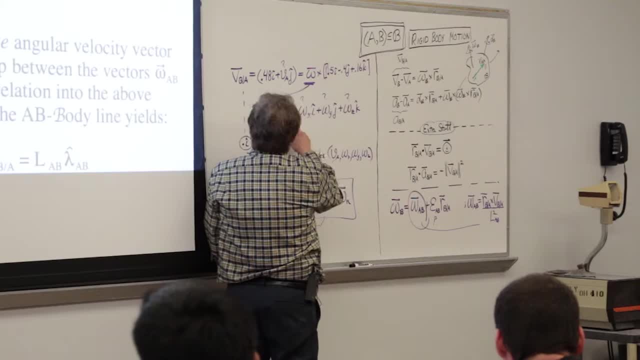 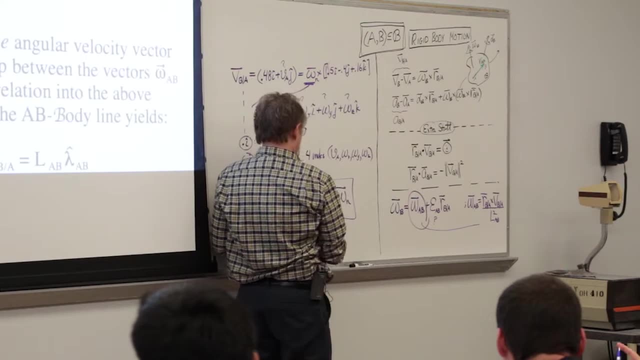 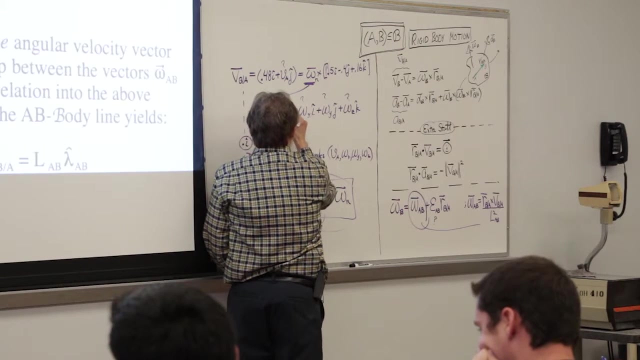 That's the only part you need. So what he said was: this doesn't in this equation right here. this doesn't have to be the entire angular velocity vector. All it has to be is this part. So okay, So all he needs is that part. 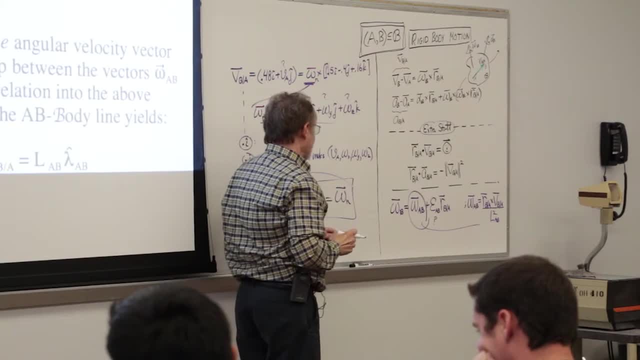 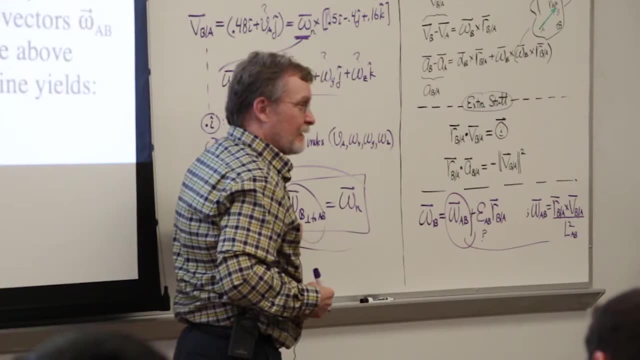 Well, It's completely unknown. So it's still three unknowns. You say: well, how does that help you? You still don't know anything about it, except you know what? Except you know that this vector called omega n is the only thing you know about. it is. 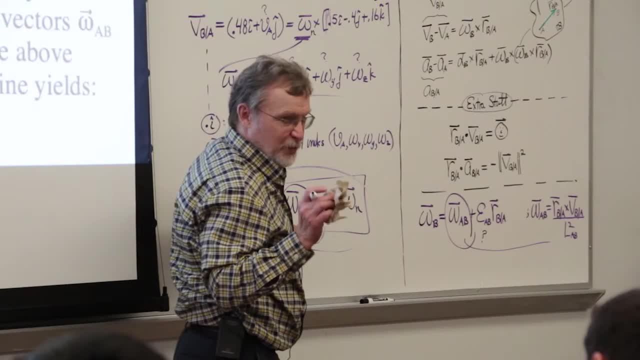 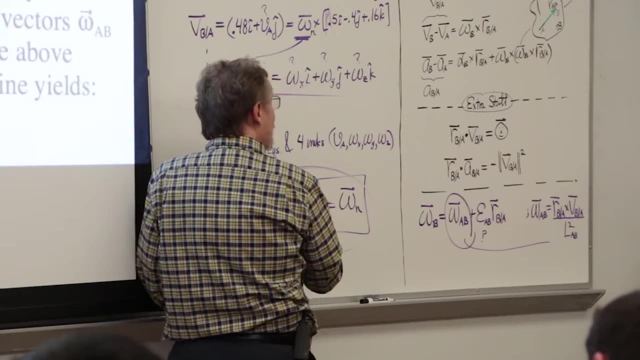 is that it's. you don't know its direction. it's a three dimension. You know it's perpendicular to AB, That's all you really know. But doesn't that fact that it's perpendicular to AB, doesn't that give you another equation? 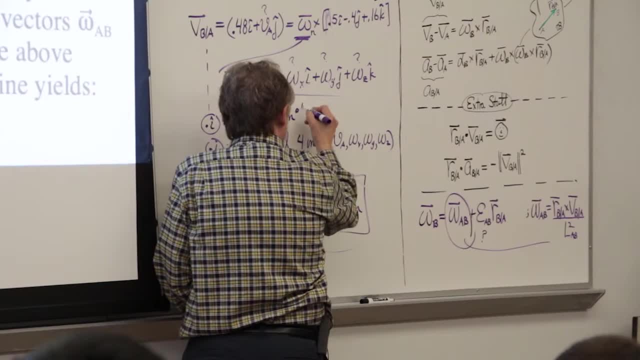 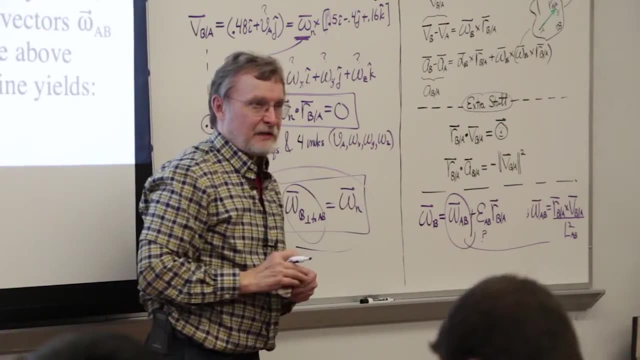 that you could write down. If two vectors are perpendicular, couldn't you write this equation Expressing the perpendicularity between those two vectors And, in point of fact, the three equations that come out of this, the three I, J, K component? 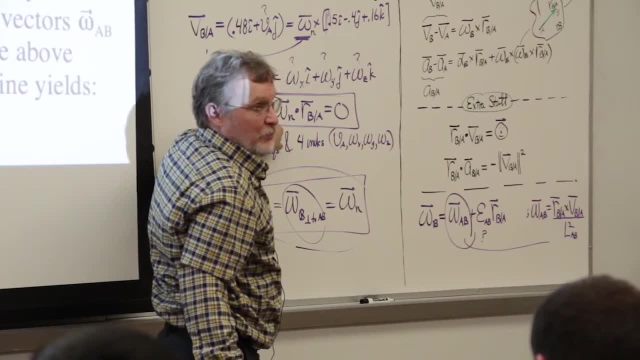 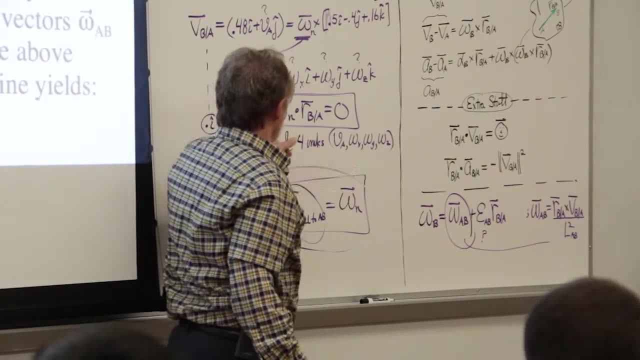 equations. make your first three equations and then this one becomes your fourth equation And what you're left with is now one, two, three, four equations to solve for four unknowns, And if you've had a chance to look at that solution, 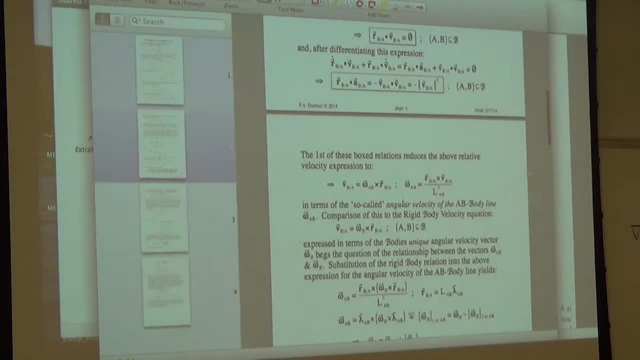 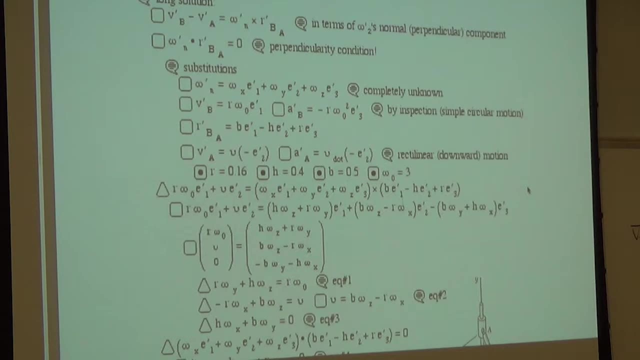 Okay, You'll see how ugly it gets. Here's where he sets up the equation on top and he's realized at this point that he doesn't need the entire angular velocity of the link. All he needs is that angular velocity of the AB body line, AKA omega sub n. 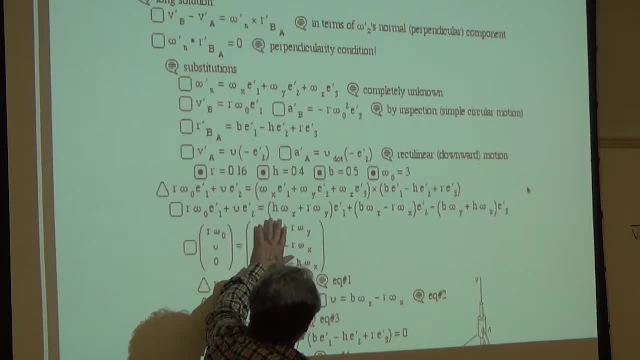 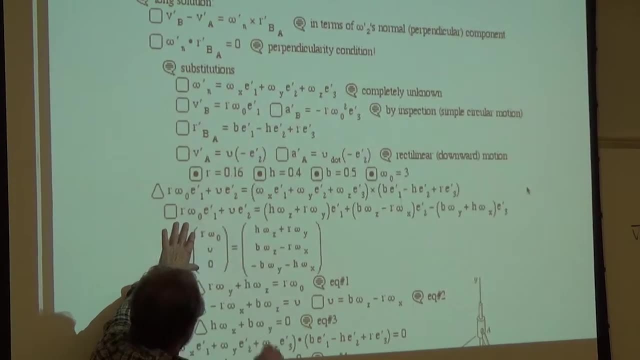 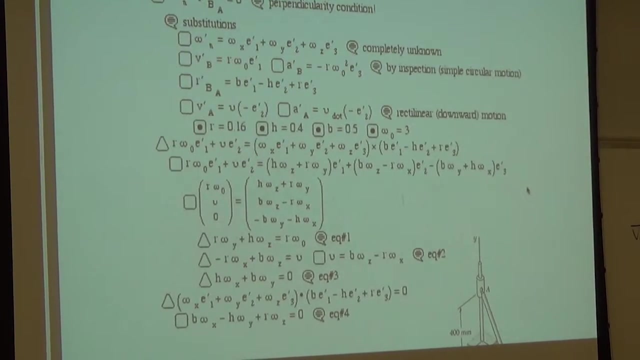 He substitutes in H and R and B are the 0.5, 0.4 and 0.16 numbers. In any case, these are the three equations that come out of the vector equation, plus three first three component equations, plus he's got the fourth equation, which is the 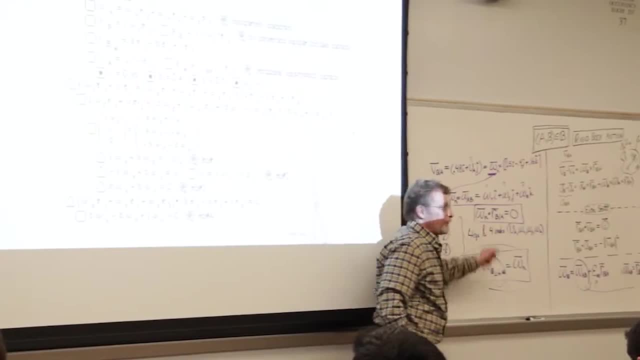 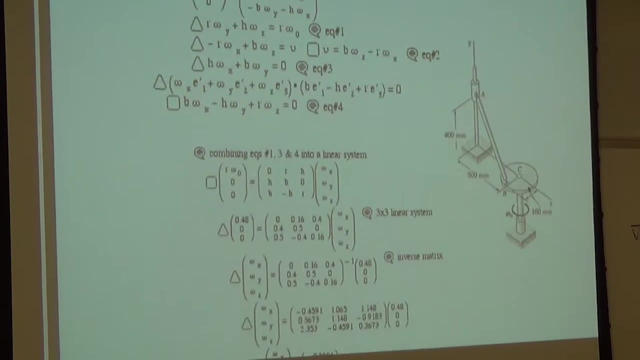 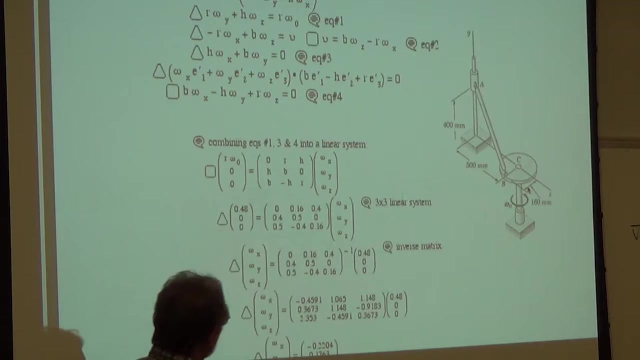 zero dot product relationship. That's this equation, right here. He then, I think, takes the first. where does he take the first, third and fourth of those equations? and he can isolate three equations containing three unknowns, And he writes it in matrix form. 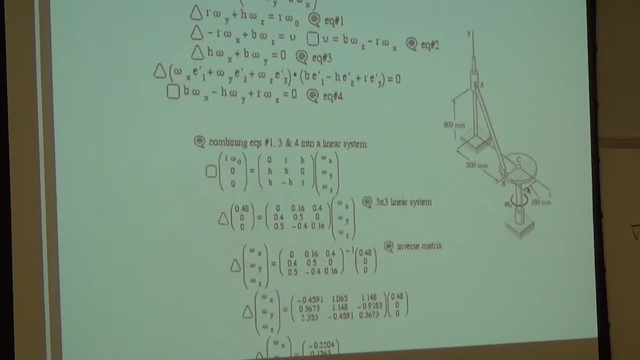 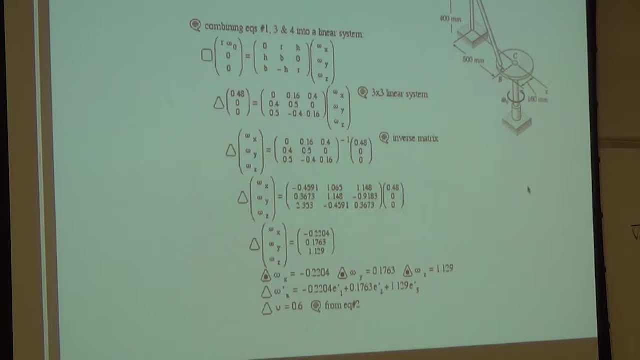 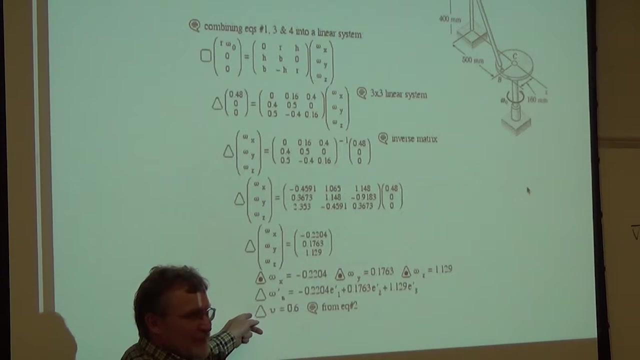 He does it matrix inverse. He solves those basically solving four equations or three equations simultaneously for three unknowns, And then he back substitutes into equation two to solve for the speed and lo and behold, he gets exactly what we got With one stinking equation. he gets exactly what we got. 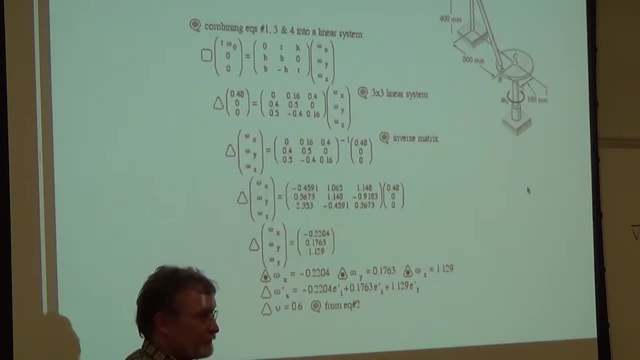 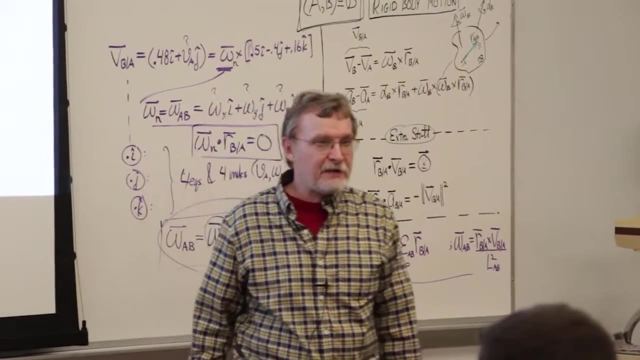 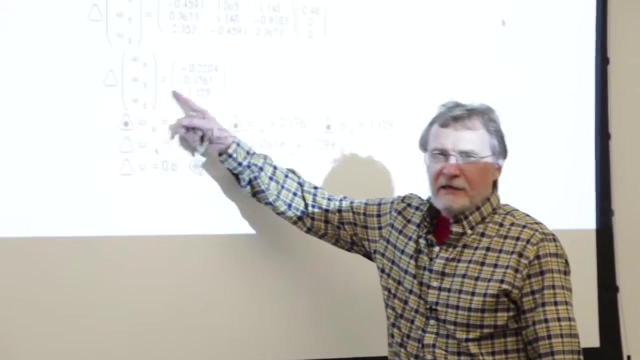 Wow, Which method would you rather go through? The one little scalar dot product relationship got us there a hell of a lot, Okay. So you might argue: well, he got something extra for his effort, didn't he? He got the. he basically was able to figure out that omega sub n vector, the portion of 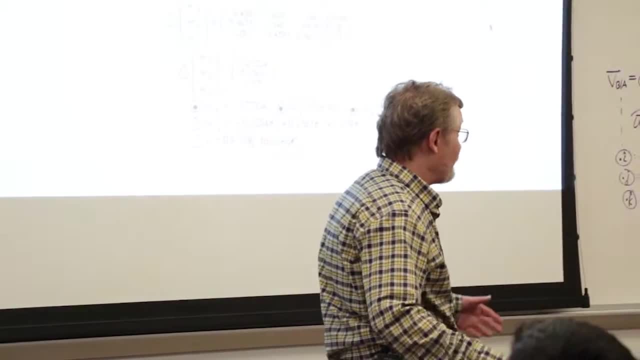 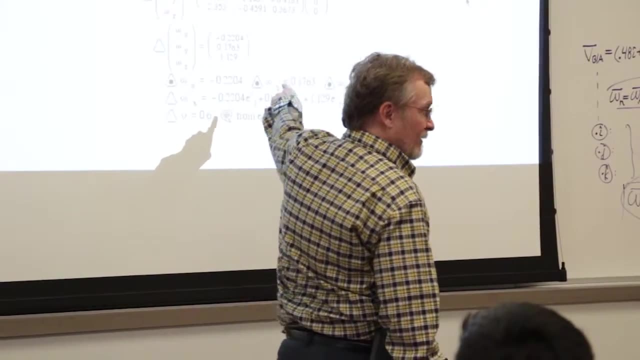 the body's angular velocity, which is perpendicular to it. And we didn't get that. We didn't even come into our, didn't even come into our assessment. But could we get that too? Yes, Because once we solve for the speed, 0.6.. 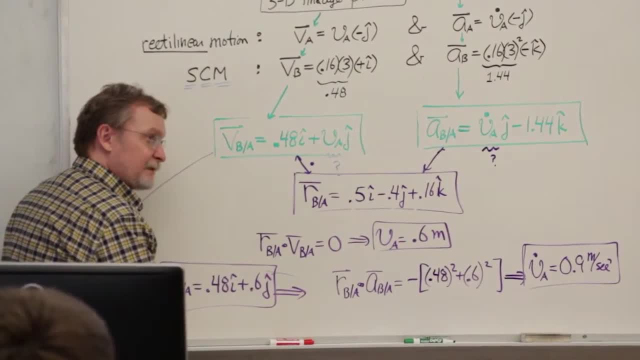 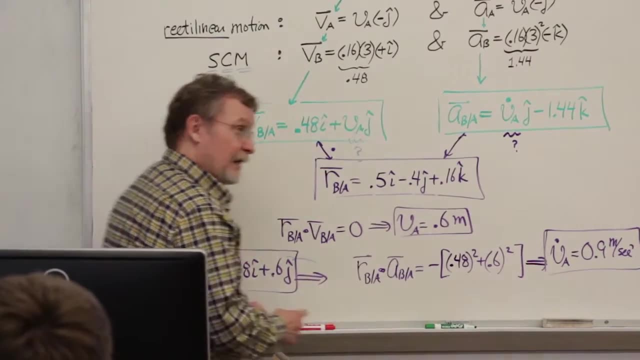 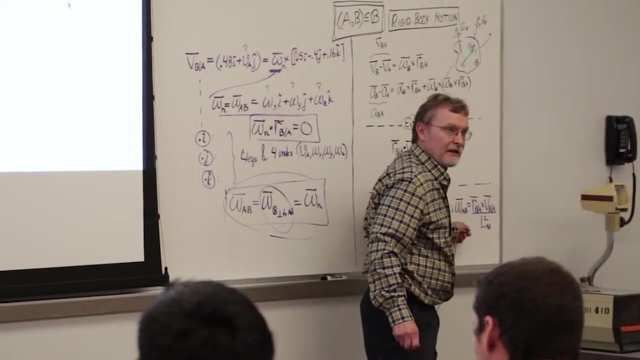 Yes, Yes, Yes. Didn't we know the relative velocity between those two points? Anybody stopping us from crossing this? with this, and dividing through by the magnitude of this square, Just take what you've got now and plug into this formula for the angular velocity of the. 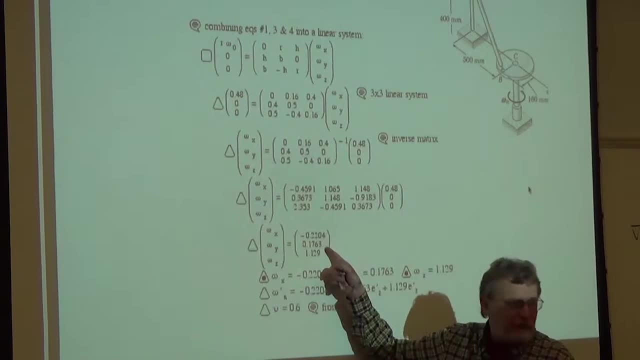 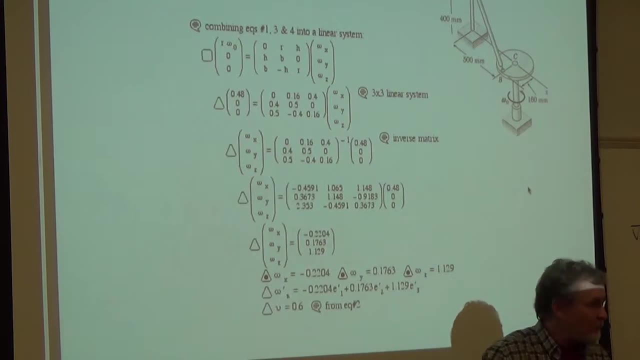 AB body line. and guess what? We get this very same thing without solving any simultaneous equations. We find VA from one equation to one unknown And then we just plug into the body line, Okay. And then we just plug into the body line angular velocity equation to get this: 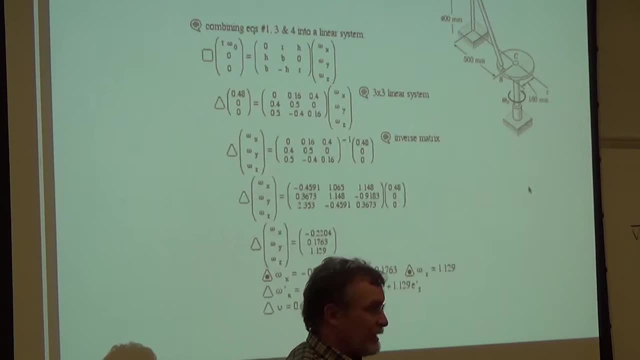 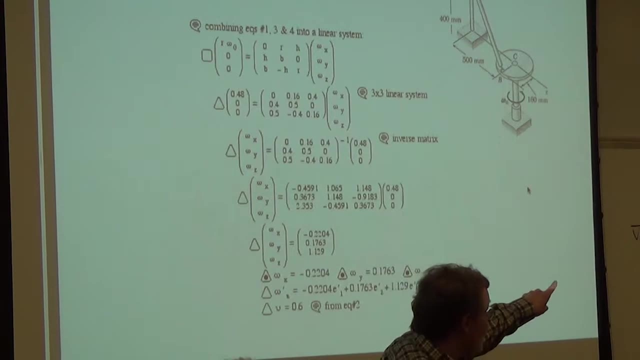 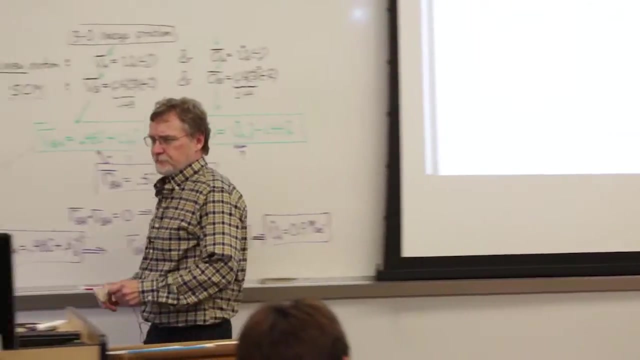 I recommend that our approach is better than his. And remember he didn't even attempt the acceleration part of the calculation. And if you wanted to go the vector route using this equation and KD bar the door, you're in a real mess then if you try to solve those equations. 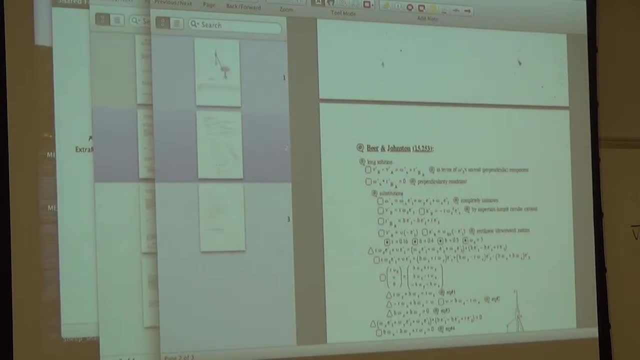 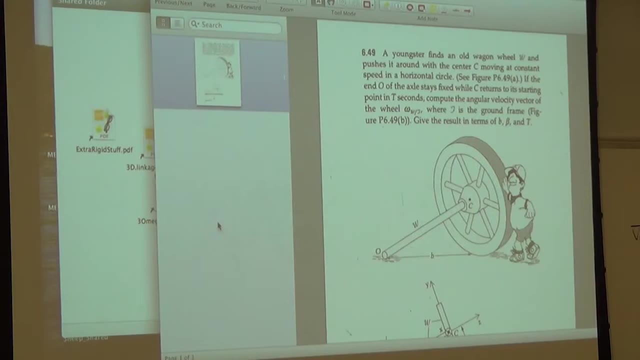 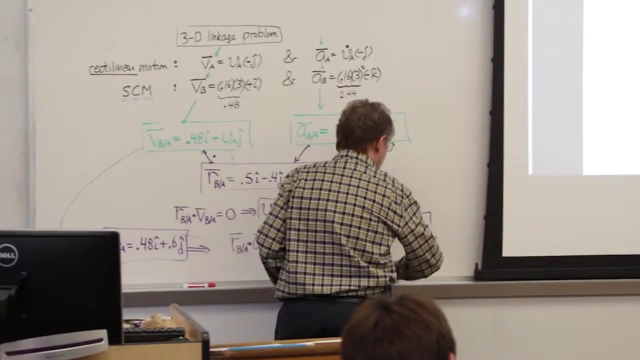 I got about three or four more minutes, So let me show you a problem. We'll get right on first thing on Friday, And it makes use of this really important fact- And here's the problem- Taken from the McGill and King textbook, which has been out of print now for a few years. 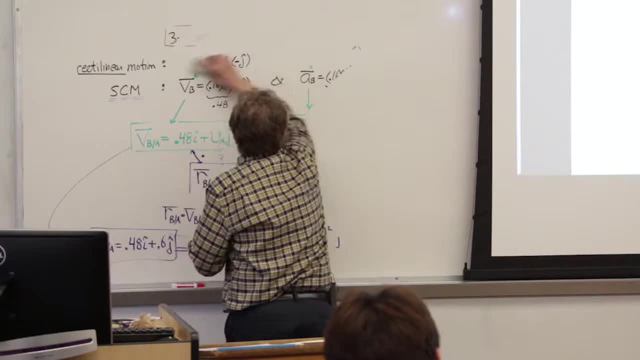 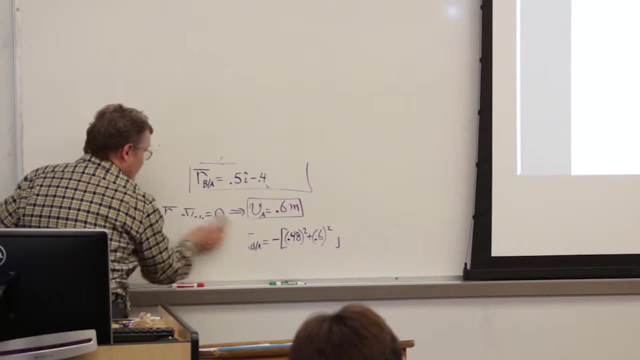 It was kind of cute in that he hired a cartoonist to do most of his illustrations, And this is a fun problem where he shows a little kid out in the field. out there He's found an old half-shaft from a chuck wagon or something like that. 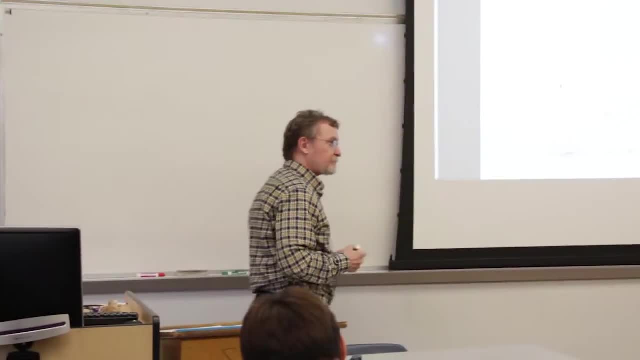 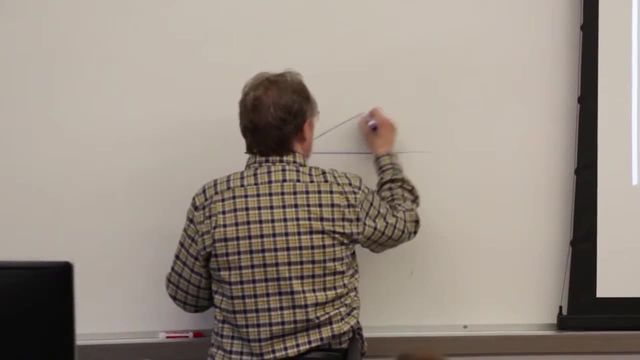 And he's amusing himself by pushing it around in a circle. All right, So, looked at from the side, what they describe, the motion that they describe, is that here's the shaft and here's the wheel itself, and they describe the end. 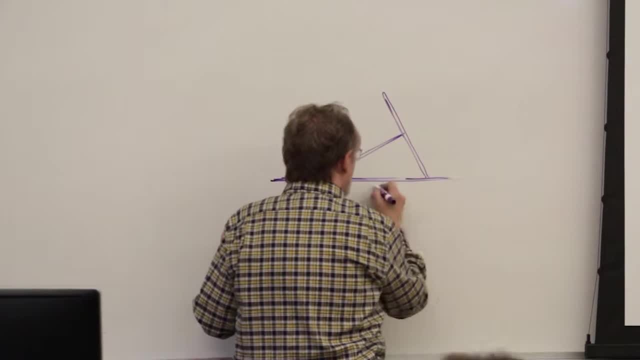 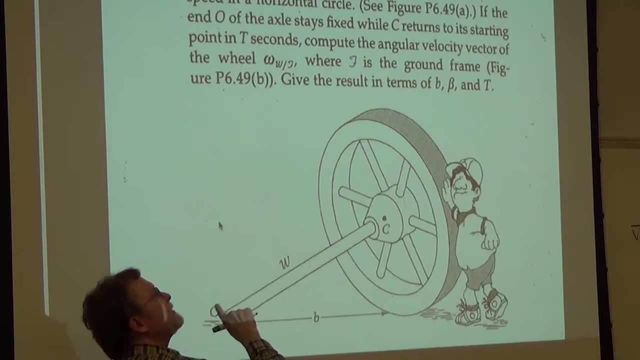 of the shaft as sort of being embedded in a little hole or crevice like that, so that this end is kind of acting like a ball and socket connector And they say: the kid just rolls it around the ground steadily like this, and I think it says something like he makes one. 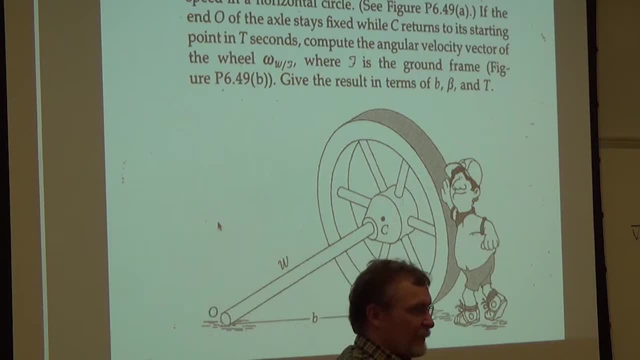 complete revolution every so many seconds. And so, given that they want to know, can you figure out the angular velocity and the angular acceleration vector for that half shaft Now, would you agree that that's a fairly complicated motion rotationally speaking? Would you agree that, to start off with, you don't know anything about the angular velocity. 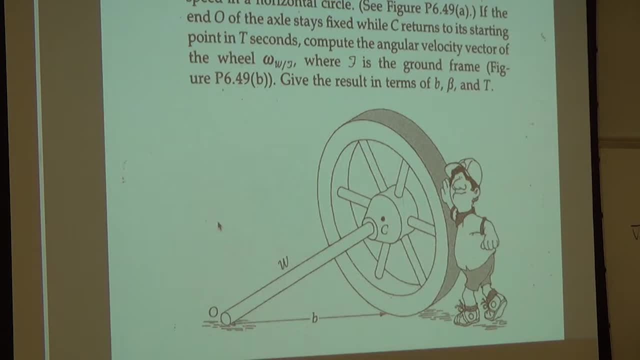 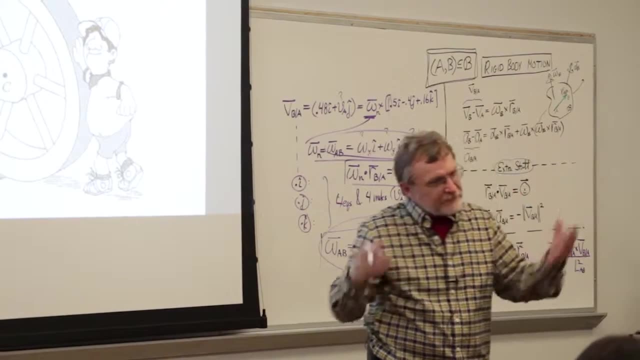 vector That in fact, would you agree that if you're looking for the angular velocity of that half shaft, it's a completely unknown vector, isn't it? So starting off, I'm saying the omega problem really has three unknowns. But watch this. 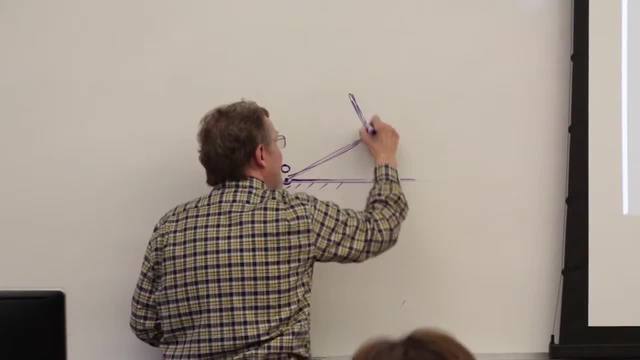 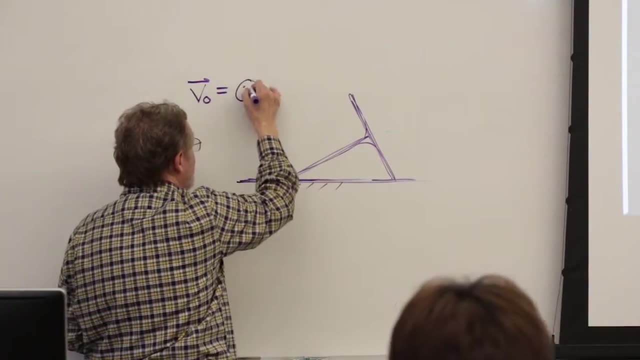 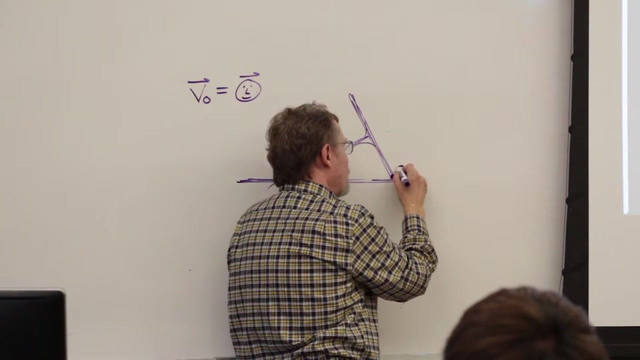 This is a rigid body. yes, Do we know the velocity of point O in that rigid body? It's clearly equal to zero. They said that the wheel is rolling on the ground, so let's look at the point right there at the bottom of the wheel. we'll call it point C. That's in no-slip. 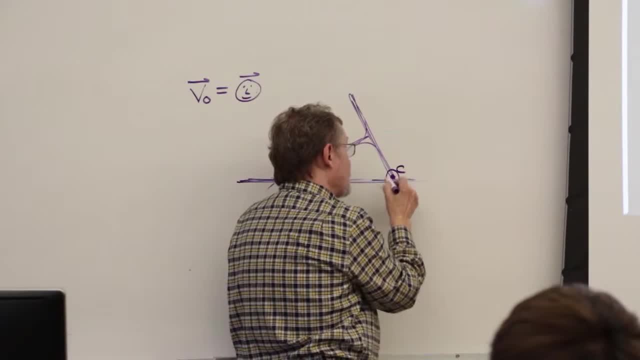 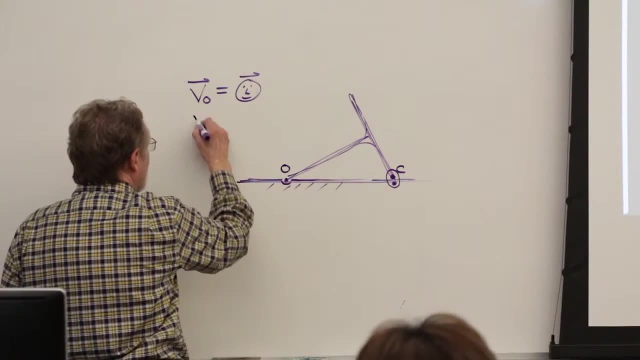 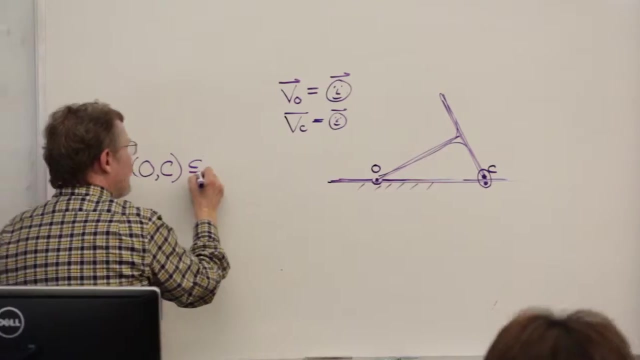 contact with the ground, is it not? Have you ever heard the words velocity match across a no-slip contact point between two bodies. So do we know the velocity of C? Follow my logic. do the points O and C? are they both points that belong to this rigid body? 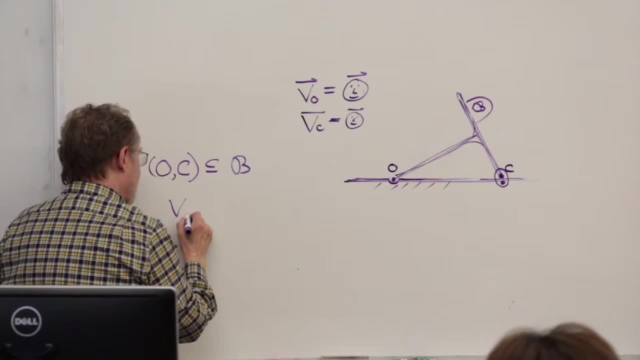 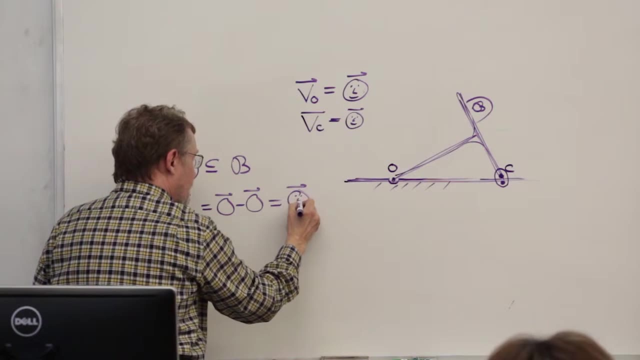 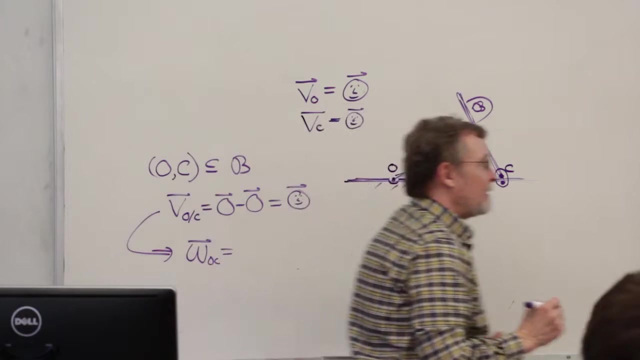 Do we know the relative velocity between those two points? Well, that would be zero minus zero, wouldn't it? Last I checked, that would be the zero vector. What does that tell us about the angular velocity of the OC body line as computed from the 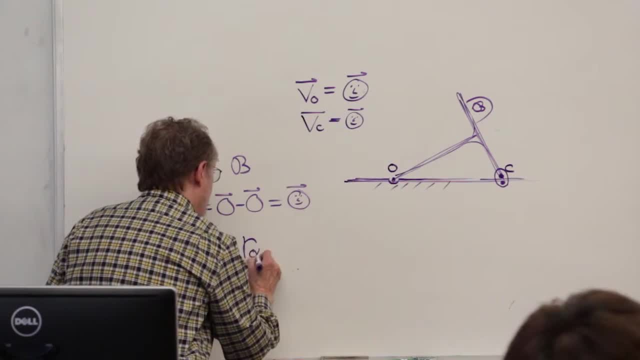 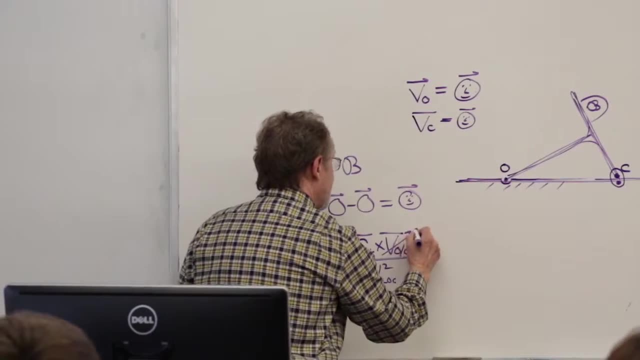 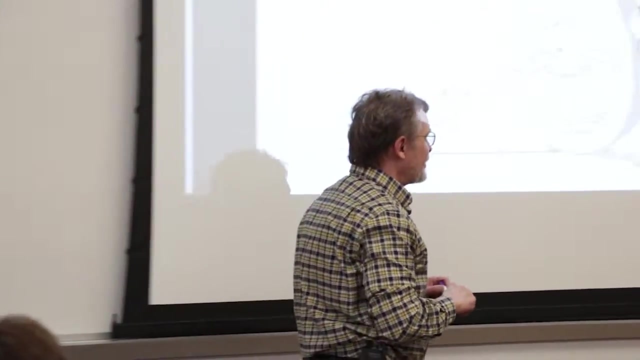 formula for such a thing: RO from C crossed, VO from C, divided by the square of the length of the line connecting them. Well, since that's zero, this is zero. So what does that equation, our last little extra bit of information, tell us That the angular velocity.